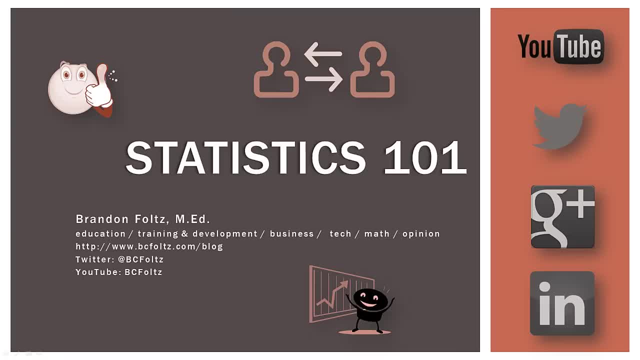 And finally, just keep in mind that these videos are meant for individuals who are relatively new to stats. So I'm just going over basic concepts, And I will be doing so in a slow, deliberate manner. Not only do I want you to know what is going on. 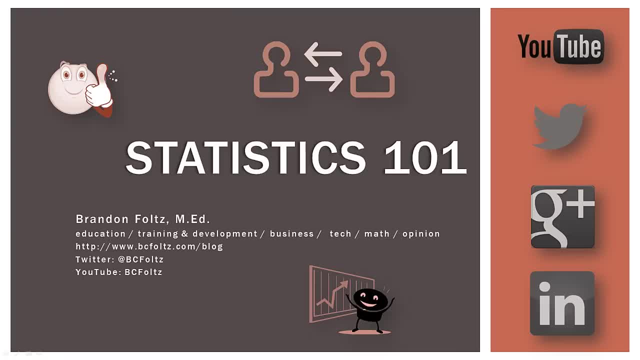 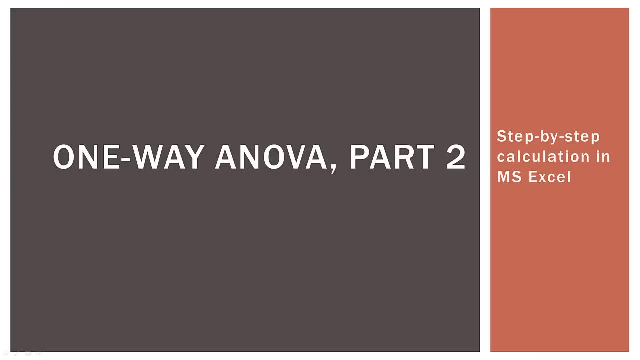 but also why and how to apply it. So, all that being said, let's go ahead and get started. So this video is part two of our larger video on the one-way analysis of variance, or the one-way ANOVA. 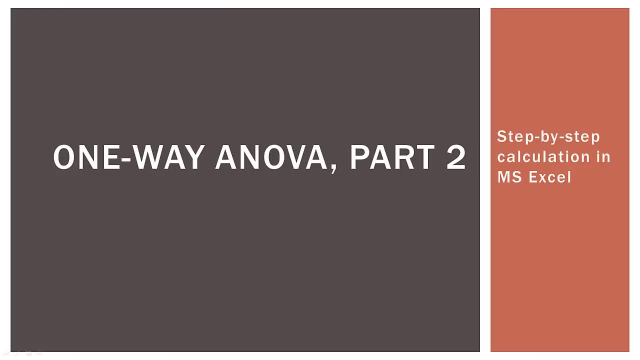 In part one we went over an example problem and really sort of took it apart and looked at how all the parts of the one-way ANOVA fit together. So in part two we're going to go into Microsoft Excel and do a quote hand calculation of the one-way ANOVA. 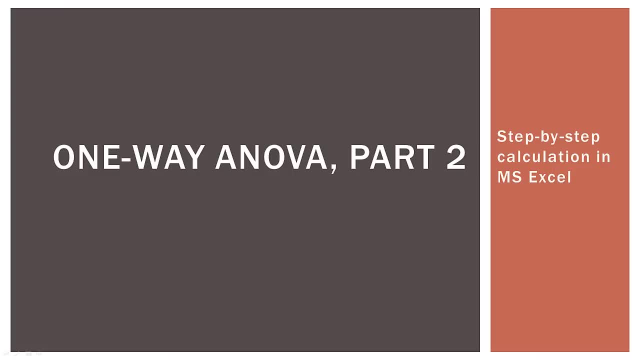 So if you're watching the video on YouTube, you can go to the description below the video and there you'll find a link to the corresponding blog post for this problem. On the blog post, you can actually download a blank version of the Excel file we're going to use. 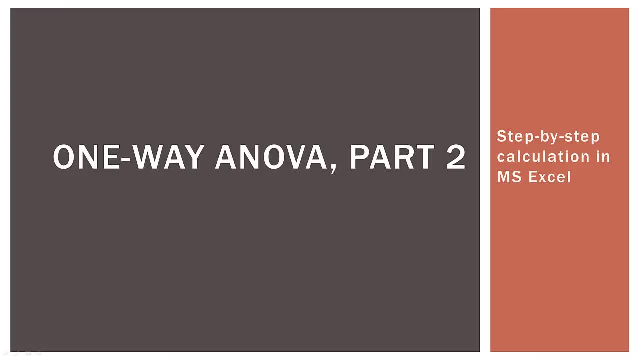 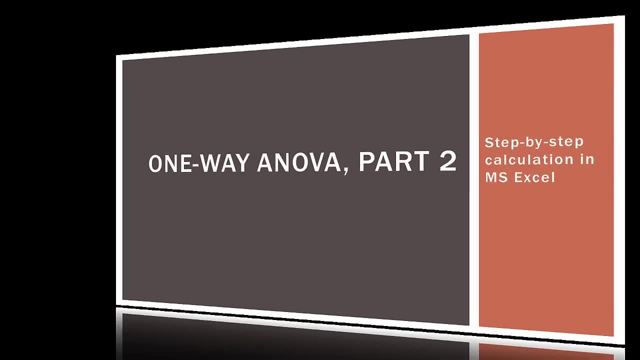 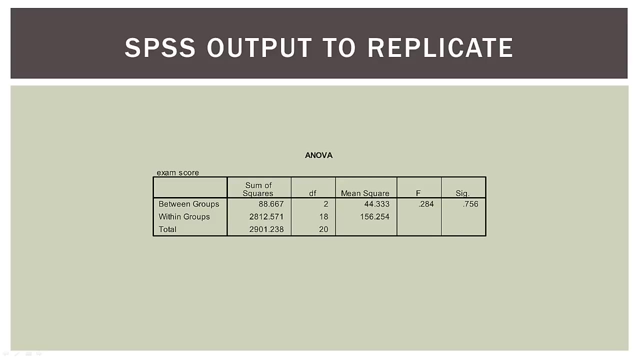 and you can follow along step by step. So, without further waiting, let's go ahead and get started on part two of the one-way analysis of variance. Now what we're going to do in Excel is try to replicate the output in SPSS. 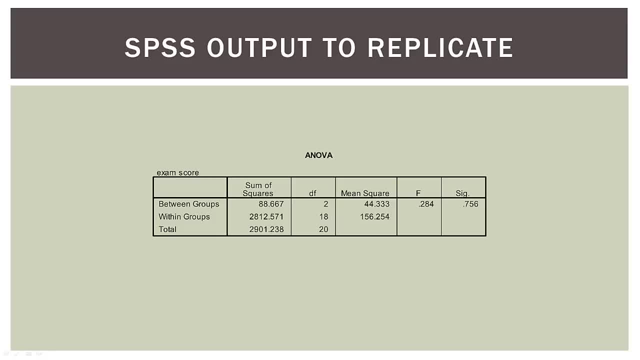 And again, SPSS is the statistical software I use in my work. So I went ahead and did our example problem in SPSS and this was the result. So we're going to go into Excel and actually try to replicate this ANOVA chart doing hand calculations. 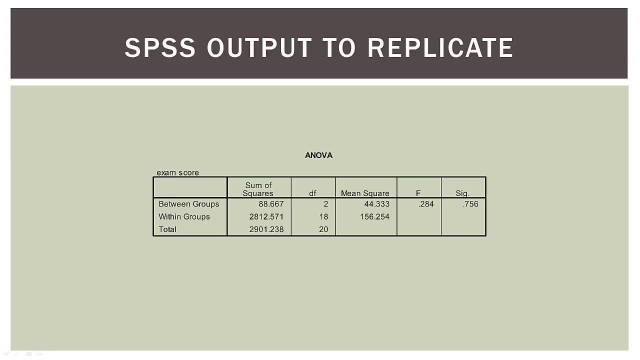 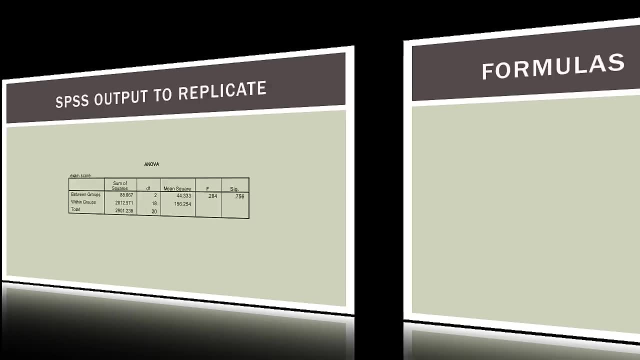 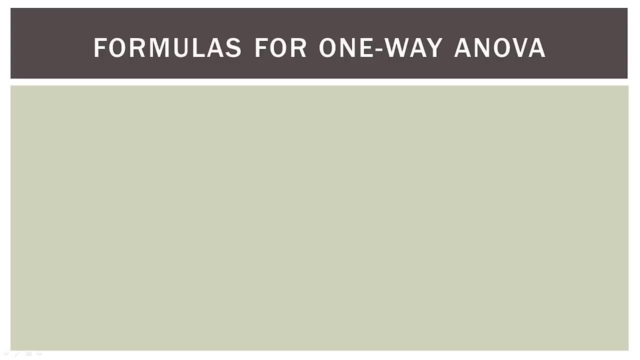 And of course I don't mean literally by hand. We're going to use Excel formulas, But in the end we want to have an example, So we're going to have a chart that looks exactly like this. Now, before we actually go into Excel, we do have to go over a few formulas for the one-way ANOVA. 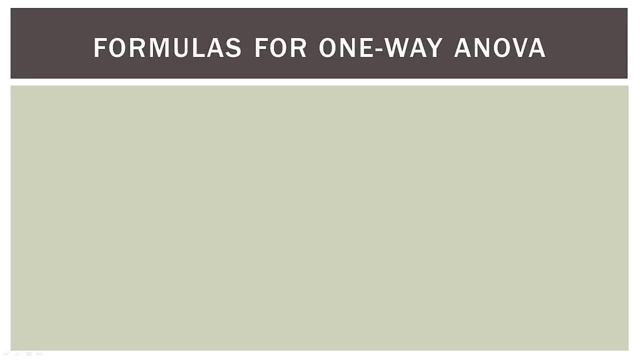 Now I mentioned before that some textbooks and some professors and classes and everything else call the same things by different names, So you may have to cross-reference what we're going to learn here with how it's presented in your class. 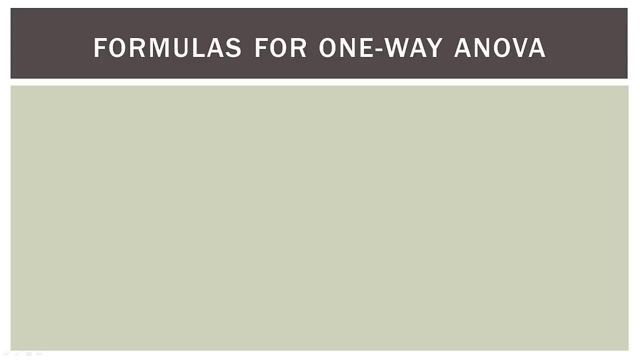 So you may actually want to have your textbook open or your notes open as we go through it. It's the same thing, but again they go by different names depending on what text you're using or what professor you have. 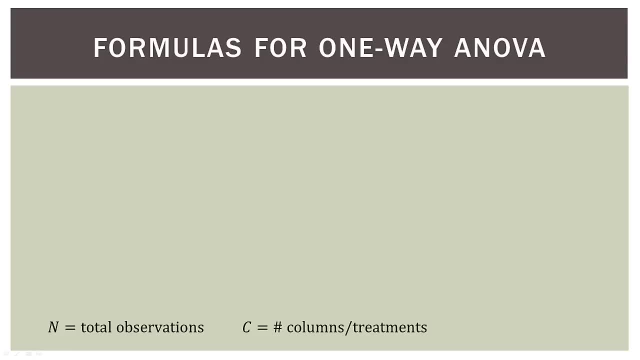 So before we do that, I just want to point out what's going to come up here in a second. When you see the variable N or the large N, that represents the total number of observations in our experiment or in our problem. 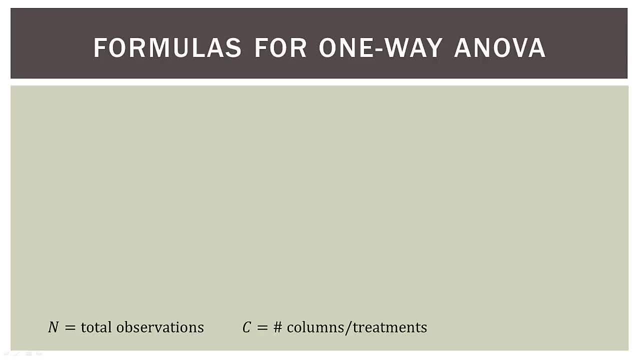 In this case it's 21,. remember Now, C is the number of columns We have in our chart, And remember, in this problem we had three because we had three years of students. So let's talk about SSC. 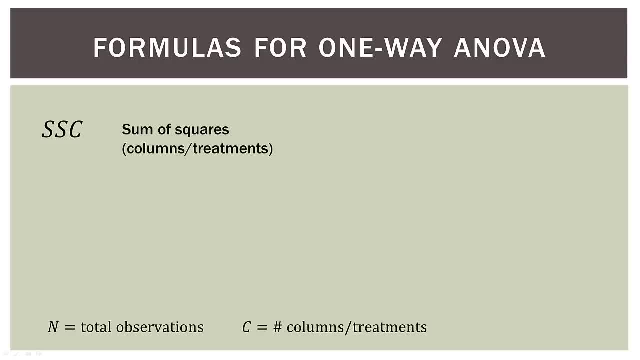 Remember that's sum of squares of the columns, or sometimes what's called the treatments. It's also the levels of our single factor we're looking at. Remember I said they can go by different names, That's what I mean. So in this case we had year one, year two and year three. 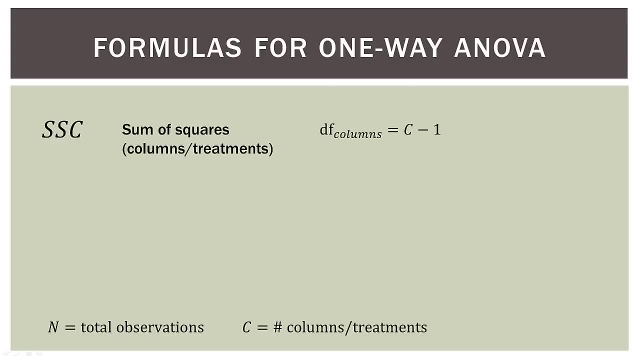 Those are our columns. Now the SSC also has degrees of freedom. Actually, all these have their own degrees of freedom. In the SSC case, the degrees of freedom of the columns is C minus one. Now the MSC is the mean squared of the columns. 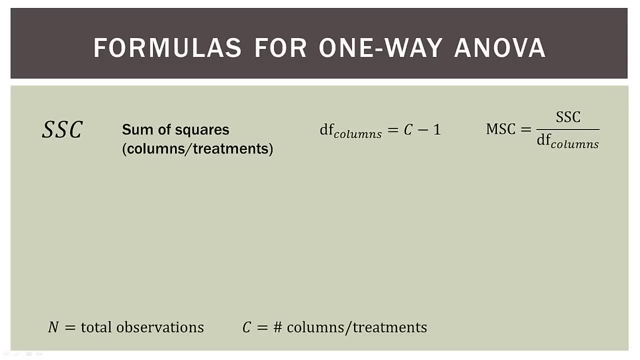 So mean square of the columns, That's MSC And that is the SSC. So the sum of squares of the columns, The sum of squares of the columns divided by its own degrees of freedom, And again, this is all very abstract until we do it. 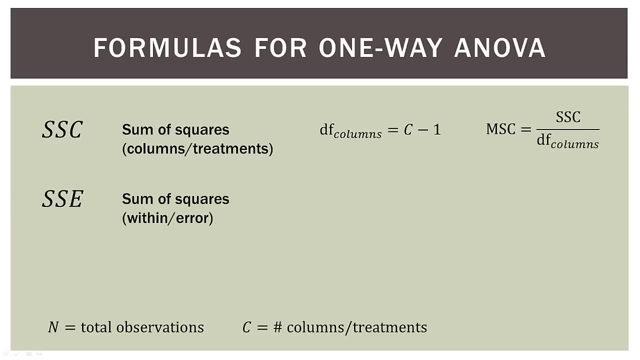 So just hang with me. So the SSE is the sum of the squares of the error, or the within each column, each individual column, sum of squares. So the SSC is the sum of squares between the columns. The SSE is the sum of squares within each column. 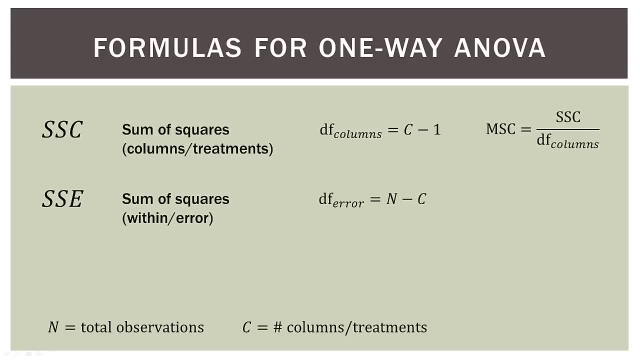 So the degrees of freedom for SSC is N minus C, And again we'll put numbers on all these here in a minute. So the MSE is the mean squared error. Now, the MSE is very important in many areas of statistics. 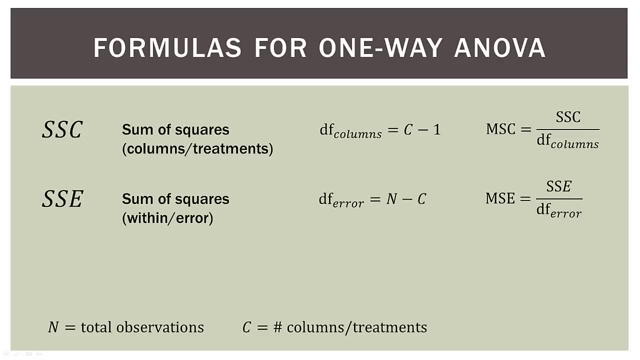 So keep that in the back of your head as we proceed. But MSC is the mean squared of the error, And that is the SSE divided by the degrees of freedom, The degrees of freedom for the error. And then we have SST, which of course is the sum of squares of the total 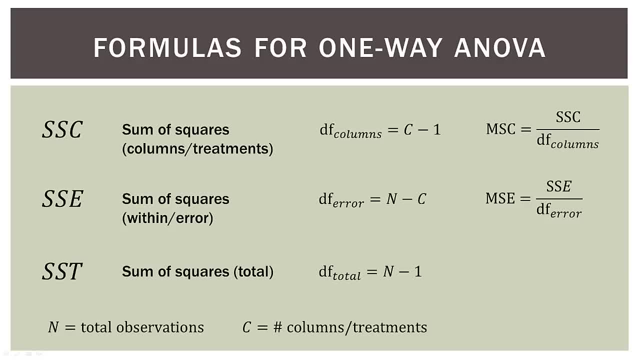 The total sum of squares, The degrees of freedom for the SST is N minus one, So the total number of observations minus one. Now, in the end we will end up with an F statistic. Remember, way back when in our F stat video, what the F statistic is. 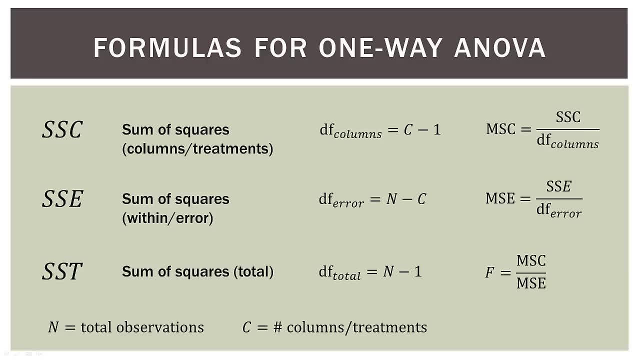 It's a ratio. F ratio is a ratio of two variances. So in our F ratio, here in the numerator, we're gonna have the mean sum of squares for the columns, which is the variance between the columns, And then in the denominator, 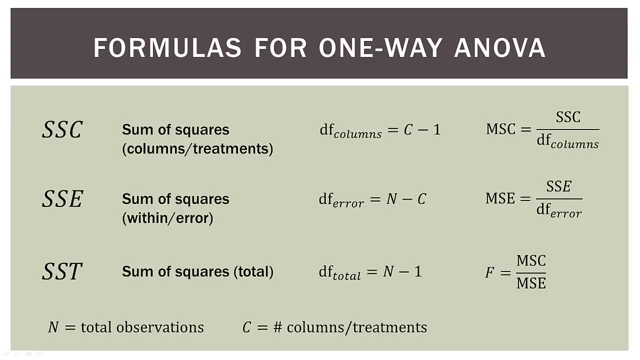 we're gonna have the mean squared error, which is the variance of the sum of squares inside the columns. So we have between the columns on top and within the columns in the denominator. That's why you will often see this as an F ratio. 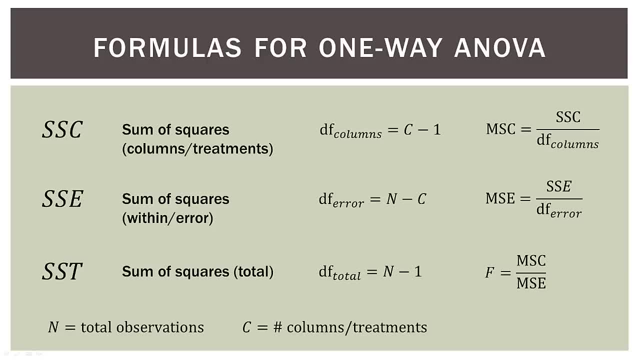 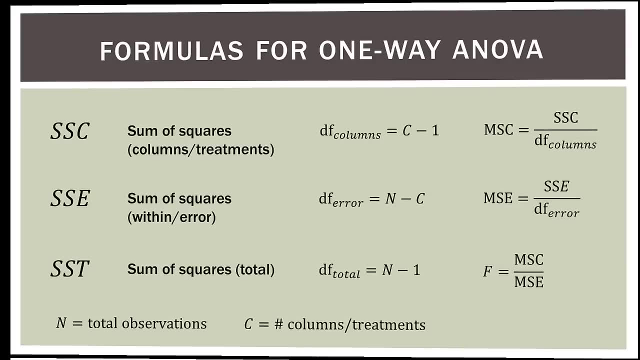 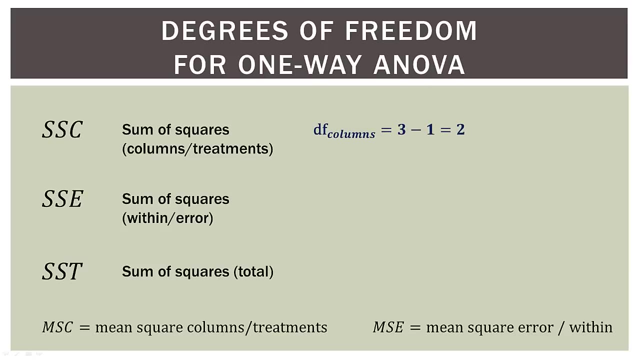 that is, between, divided by within, Between the columns, divided by the variance of the data within the columns. So let's go ahead and actually put some numbers in here. Let's find our degrees of freedom first. So remember, the degrees of freedom for SST was C. 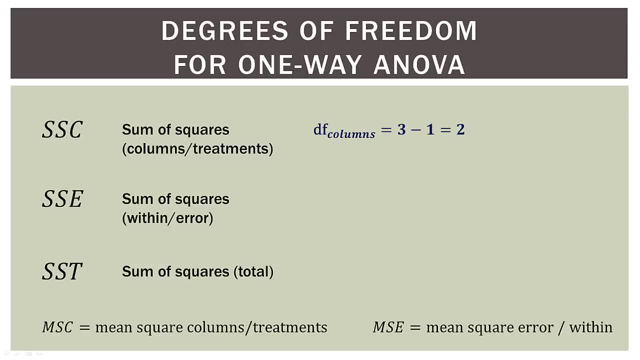 the number of columns minus one. So in this case it's three, because we have three columns minus one, which equals two. So the MSC equals the SSC divided by that degrees of freedom, which is of course two. 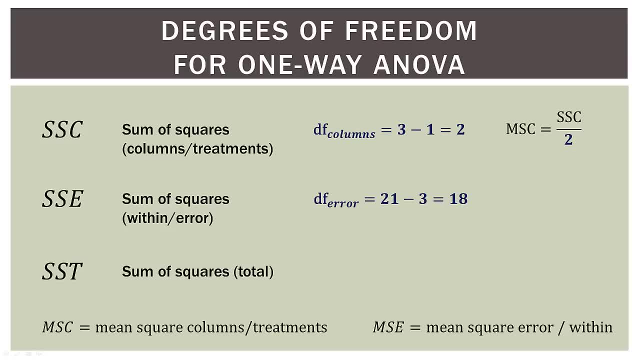 Now for the SSE. the degrees of freedom for the SSE was N minus C, So N is 21,. that's the number of overall observations minus three, which is the number of columns. So that is N minus C. 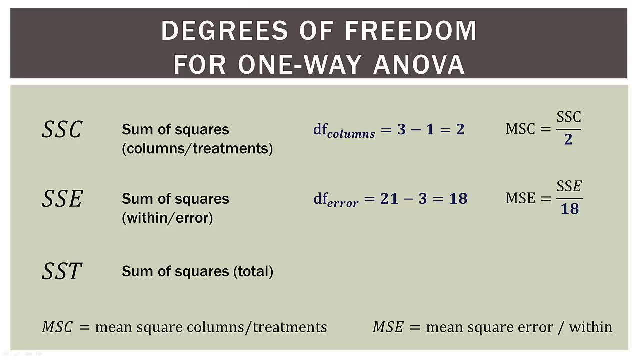 So that is 18.. So our MSC equals the SSE divided by that degrees of freedom, which is 18.. Now the degrees of freedom total, the SST, is N minus one, So our overall number of observations minus one. 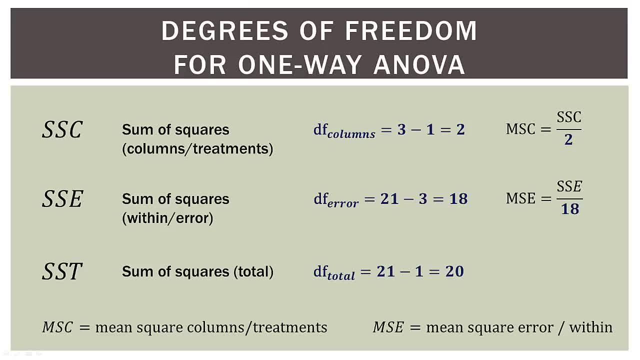 which, of course, is 21 minus one, equals 20.. Now our F ratio remains the same. It is still the MSC divided by the MSE. Now let's go ahead and go into Excel and figure out the SSC and the SSE. 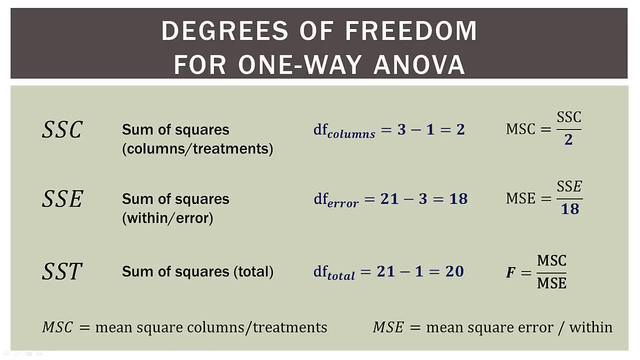 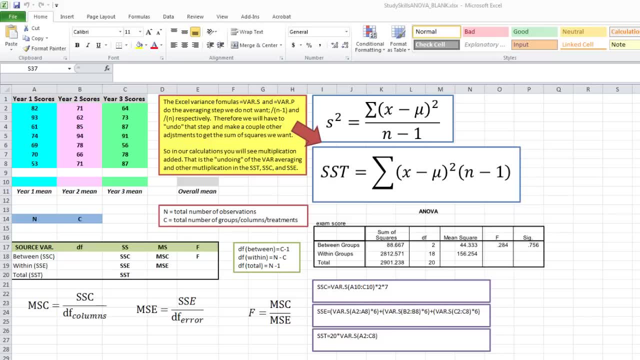 which will allow us to find the MSC and the MSE that we need to do this problem. So here we are in Excel where we're gonna do our hand calculation of this ANOVA problem. But before I give you a tour of our spreadsheet here, 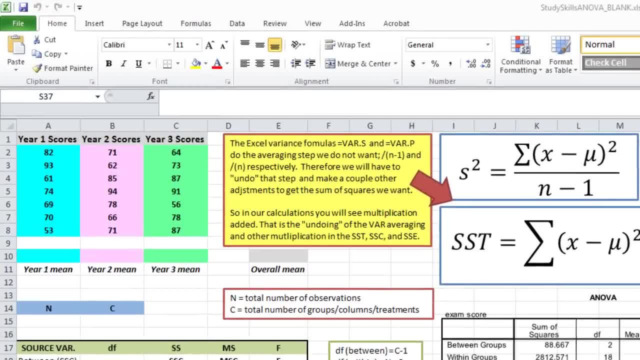 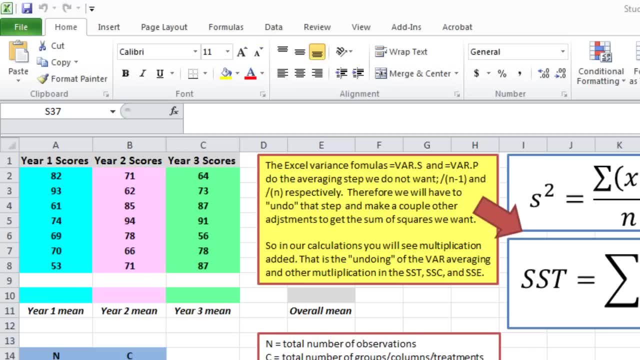 I'm gonna draw your attention to the yellow box up here at the top. Now, remember, we're gonna need the sum of squares. However, Excel does not have the sum of squares. it does not have a sum of squares formula. So what we're gonna do is we're gonna use 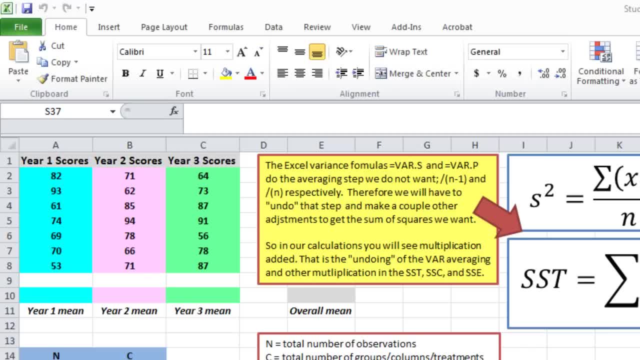 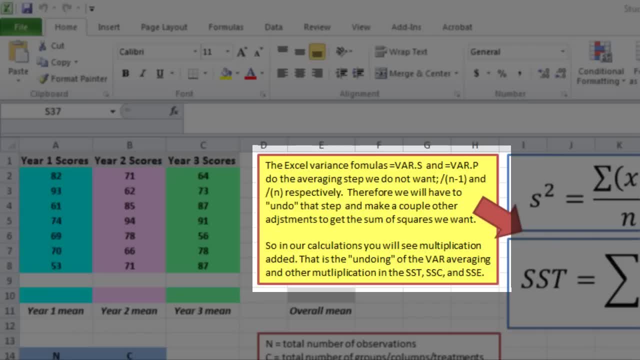 the variance formulas and then alter them a bit. So the Excel variance formulas, which is vars, and varp, which is sample variance and population variance, do the averaging step we don't want. So the sample variance will divide by N minus one. 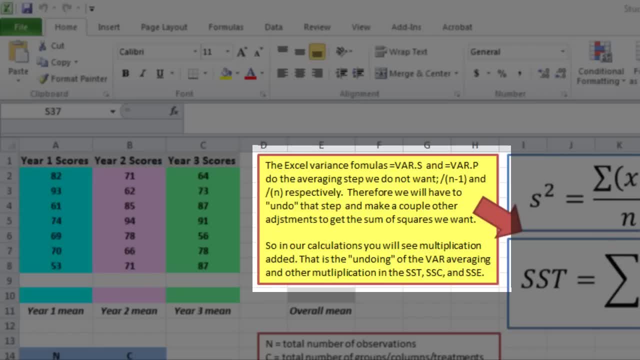 and the population variance will divide by N. Therefore we will have to sort of quote undo that step and make a couple of other adjustments to get the sum of squares we want. So in the calculations we do, in the formulas we use, 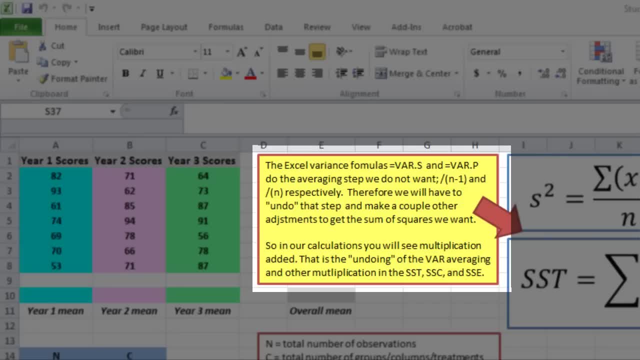 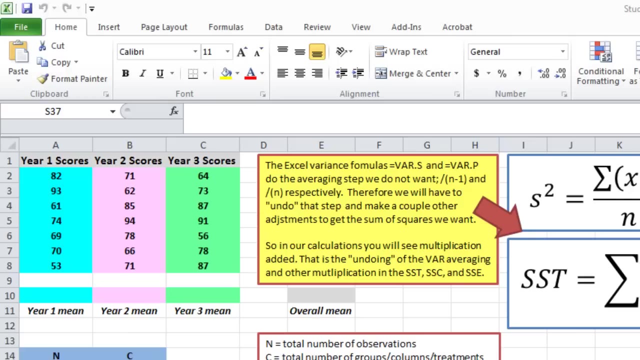 you will see multiplication added in. That is the undoing of the variance averaging and other multiplication that's in the SST, the SSC and the SSE. So what I'm saying here is that some of this you're just gonna have to take on faith. 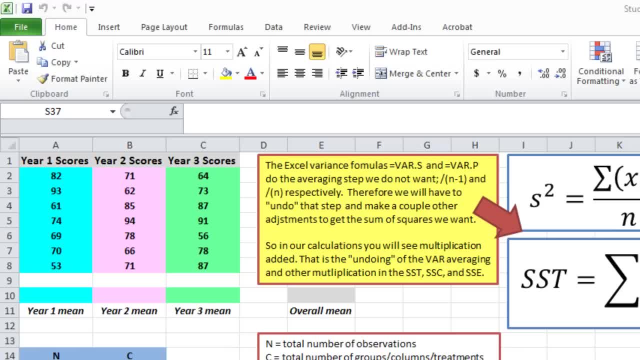 And I hate saying something like that, and I hate saying something like that in a math video, but that's just the way it is. I did not go over the individual SST, SSC and SSE formulas because I thought your face would glaze over. 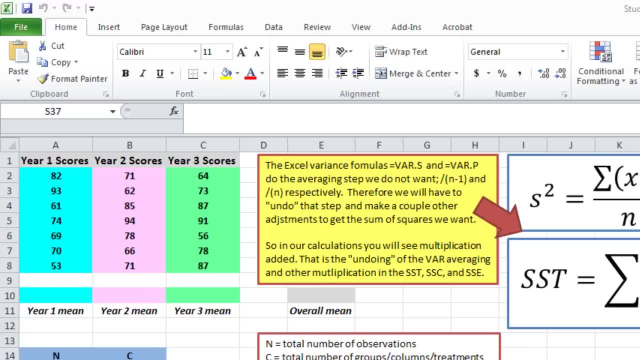 any more than it already is, and you can find those in your books. However, I will try to point out what each component is when we put in the formulas. Okay, so that's sort of my little caveat here. Now, on the top left, you will see our chart. 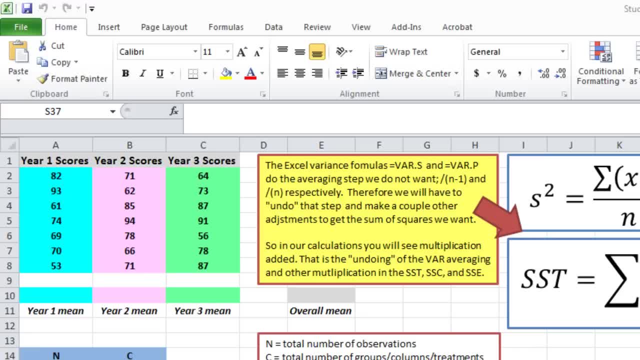 our data as we had it in the PowerPoint portion. So we have our year one scores, our year two scores and our year three scores. Nothing much surprise there. And then we have a column summary. so the mean for year one, year two and year three. 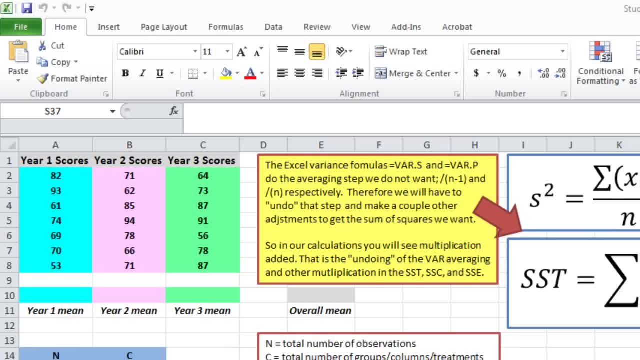 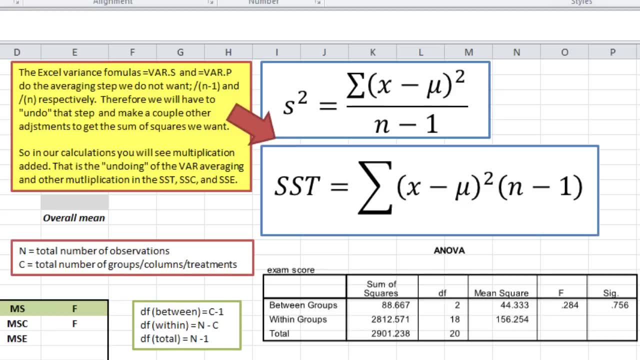 and then we have the overall mean there in the middle. Now, over on the right-hand side, I just put the formulas for the sample variance and the sum of squares we're gonna be doing, If you're really not interested in the formulas that much. 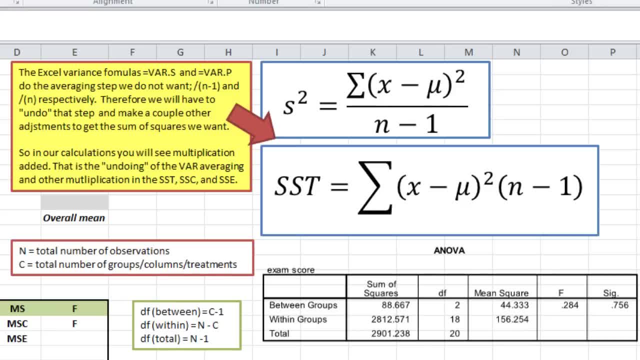 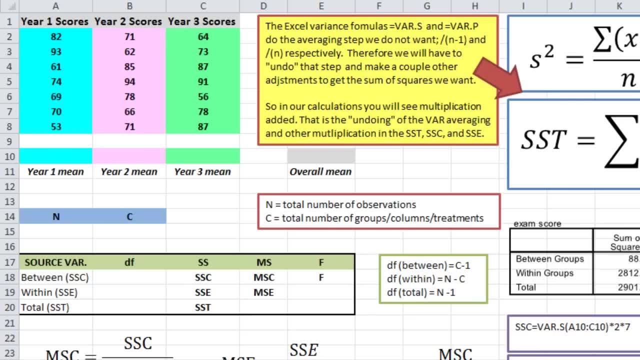 just ignore those two blue boxes up there in the right-hand side. Now, if you look below our data, you'll see N and C. Well, N, remember, is gonna be the total number of observations we have, which, in this problem, of course, will be 21.. 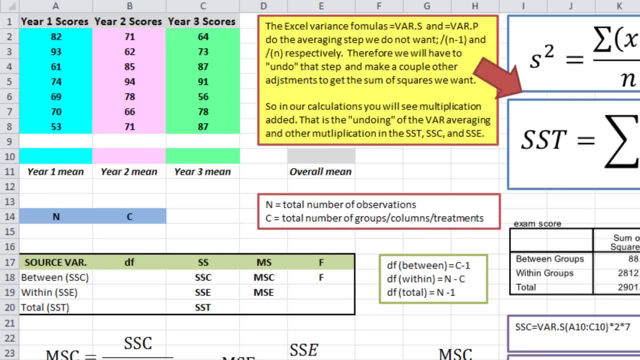 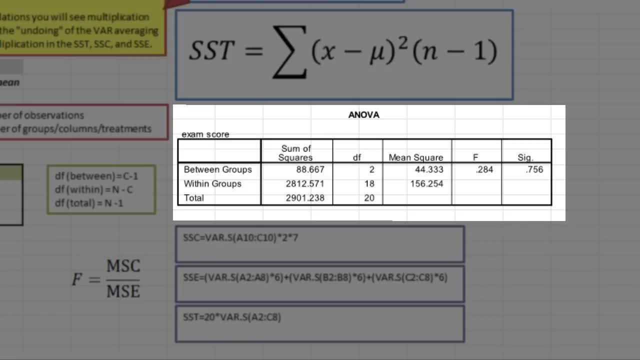 C is the number of groups or columns or treatments we have. So in this problem it will be three. Over on the right you will see the SPSS output for this problem. So what we're gonna try to do is replicate. 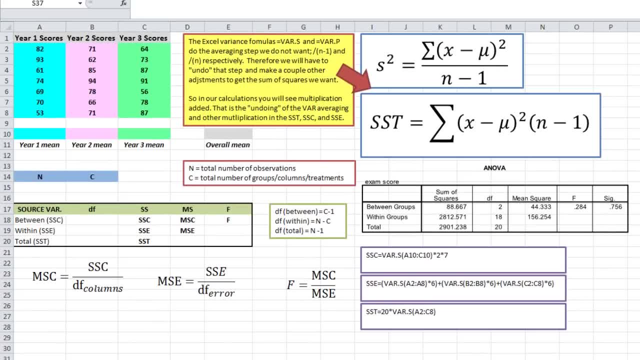 that little chart over there on the left-hand side where we have the green hexagon and then the SPSS pattern and then the SSC, SSC, SST there in that chart. So we're gonna try to make that chart on the left. look like the SPSS output over here on the right. 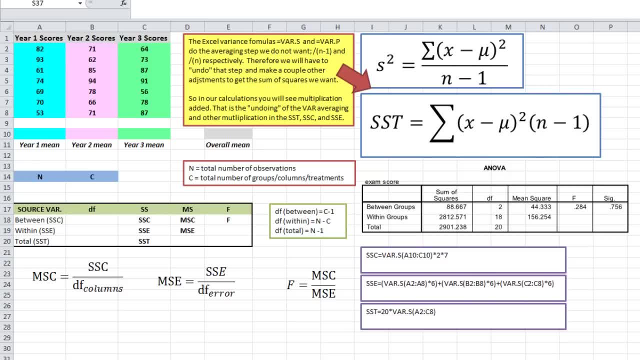 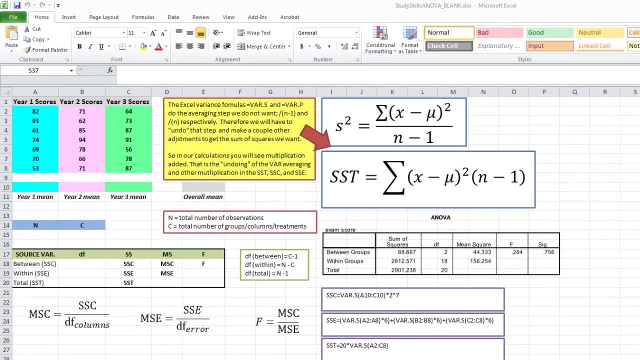 And of course, we will actually do this problem in Excel using its ANOVA. So we're gonna have three versions or three outputs of the exact same thing to make them all match. Now, everything else on here is pretty much a hint. 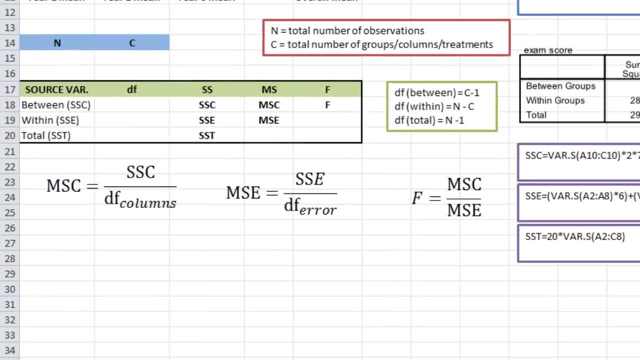 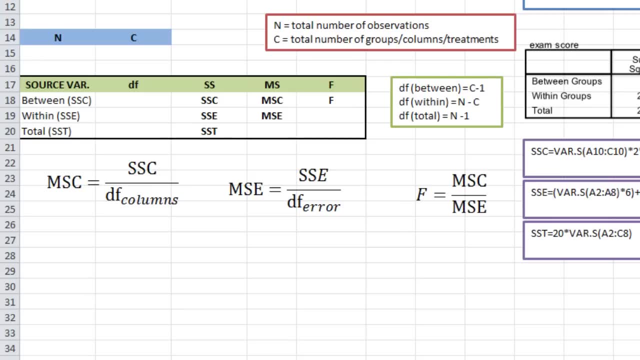 so we don't have to go back to PowerPoint to find these formulas. So below there on the left-hand side you will see the MSC, the MSE and the F ratio, And again, those just come from our slides we already had. 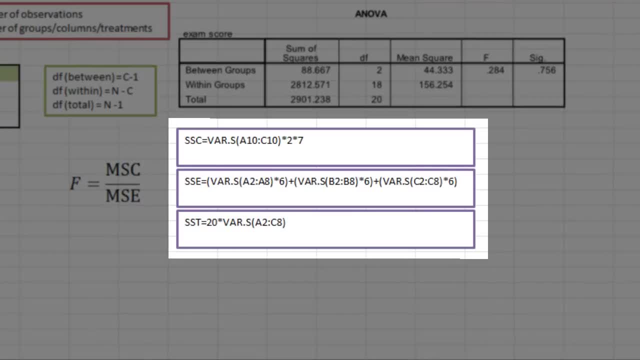 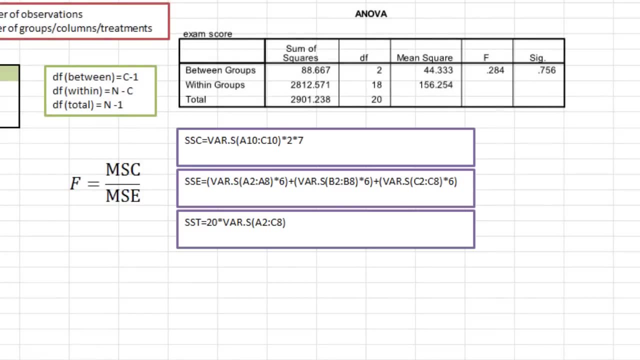 Now in the purple boxes on the lower right, those are the formulas we're gonna use to actually find our sum of squares. So I will explain those further when we get to that step, but I just wanted to put them here, sort of in a text format. 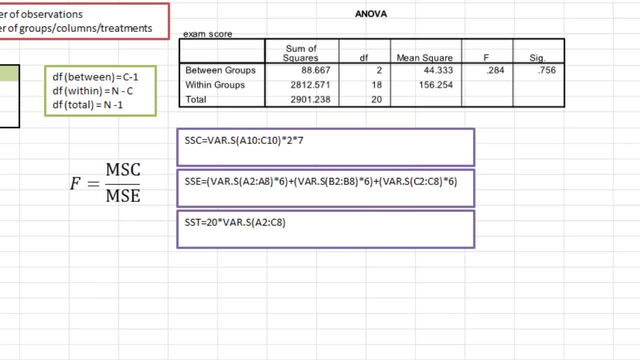 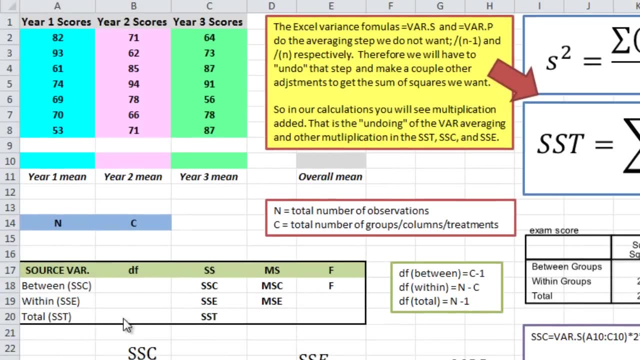 so you can copy and paste them into the proper cell. So let's go ahead and do that. So let's go ahead and do some actual calculations and put in some data. So the first thing we're gonna do is we're gonna go over to the N and the C boxes. 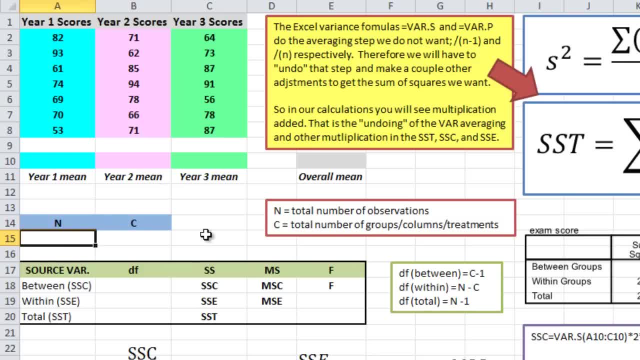 over here on the left-hand side. So this is easy. So our N in this case is 21.. So we're gonna go ahead and put 21 there. That's the number of observations we have, And then C is the number of columns, which is three. 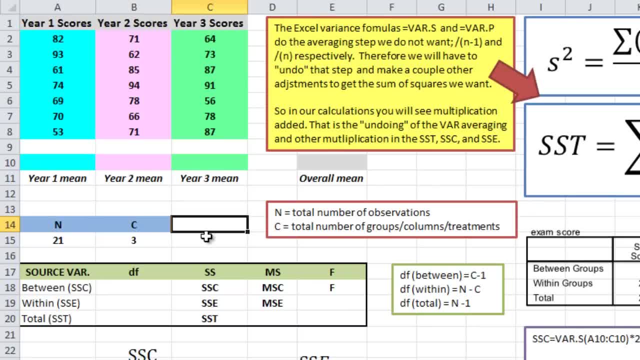 So we'll go ahead and do that. Now the next thing I wanna do is find the column means. So we'll go up to the year one mean box, which is the bottom of the year one scores, And then we'll use the average formula. 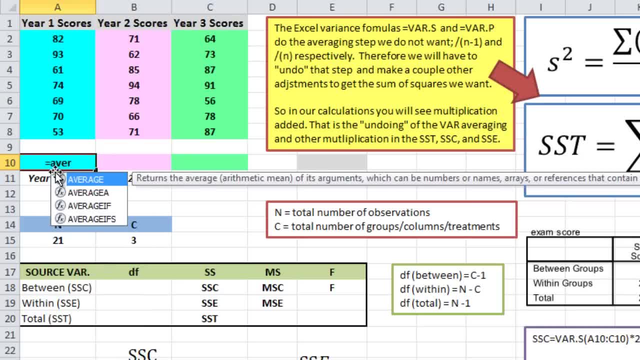 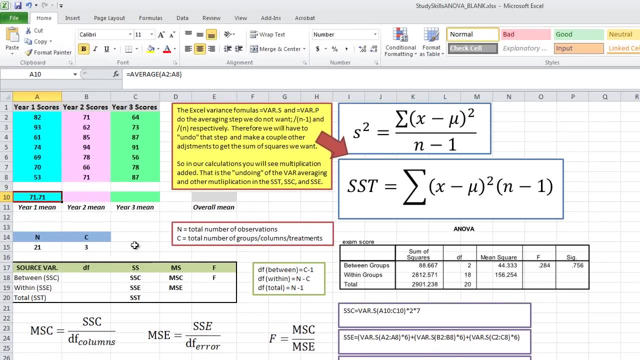 So we'll type equals average And then actually go ahead and begin filling that out. Now we'll just select all seven of those scores in the year one column, Close parentheses And there we go. So this is 71.71, which is what we had in the PowerPoint. 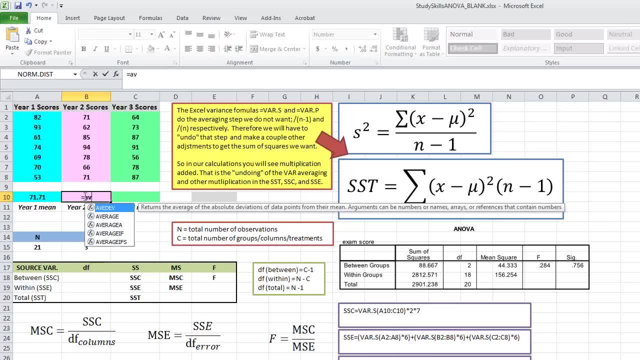 Now we need the mean for all three columns. So we'll go ahead and do the same thing for year two And we'll go into the same thing for year three. In case you're wondering, I don't drag across because it takes the color with it. 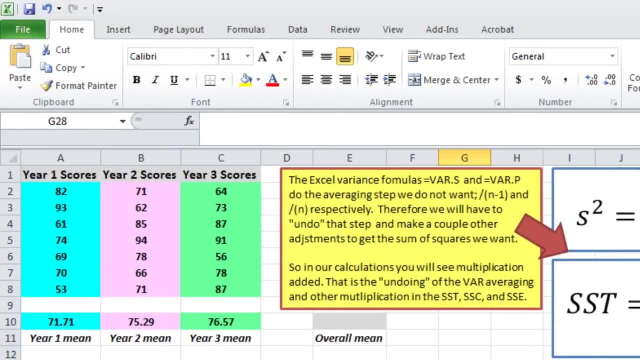 So they would all be blue if I dragged across. Okay, so we have the column mean for each of the student years, So 71.71 for year one students, 75.29 for year two students and 76.57 for year three students. 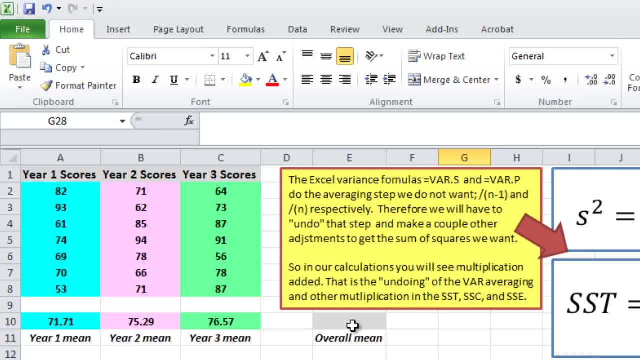 Now we want the overall mean, which is in this gray box here below the yellow box. So again equals average, And then we'll select all 21 scores in our data and hit enter. So now we have our overall mean of 74.52.. 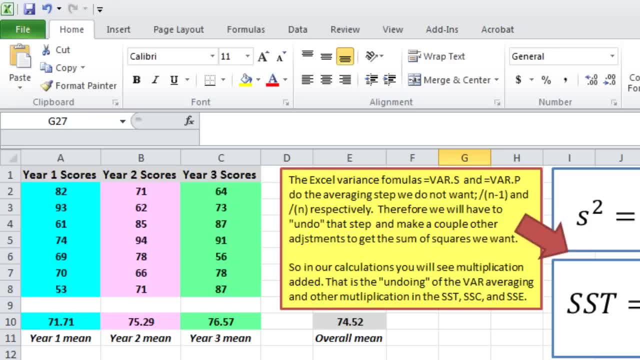 So, again using Excel, we did hand calculations of all three column means and the overall mean, which, of course, we know we need to do this type of problem. Now let's go ahead and go down to our chart over here on the lower left. 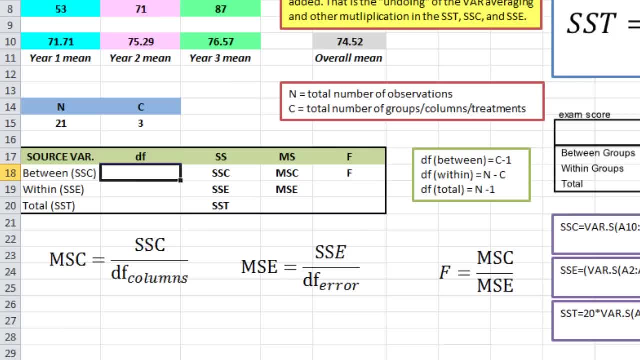 Let's go ahead and find the degrees of freedom for each source of variance. So, remember, we have column variance, so we're between the columns, We have within each column variance, and then we have the total sum of squares, the total variance. 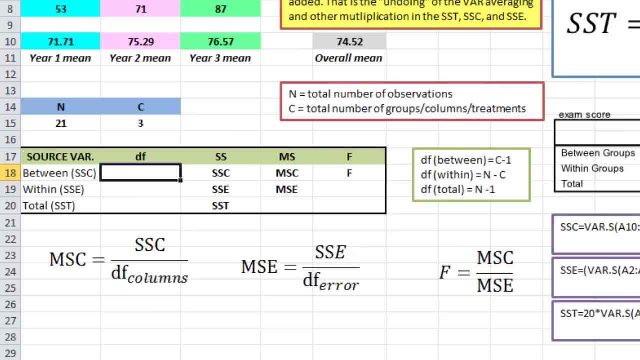 Okay. so remember that for the SSC we can see this sort of over here on the right-hand side. So degrees of variance, Degrees of freedom, between which is the same thing as SSC, is C minus one, So we could say equals C. 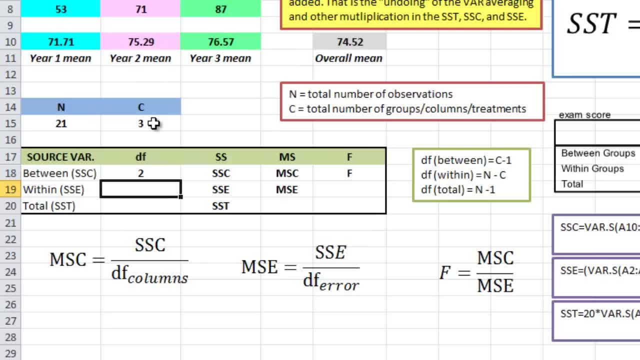 which is this cell right here, minus one, And of course that is two. Now we need degrees of freedom for within, So that is N minus C And you can see that little box on the right to help you sort of cheat a little. 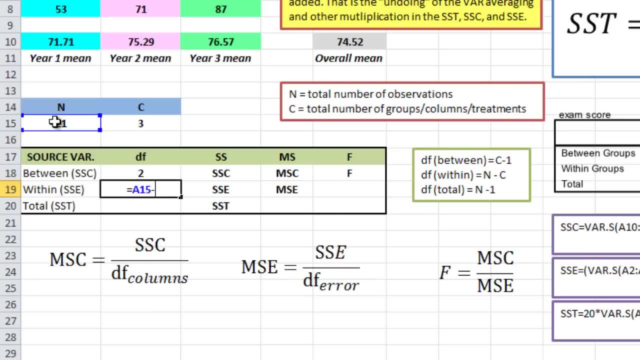 So equals N, which is that cell, minus C, which is that cell, And that gives us 18 degrees of freedom. Now our total degrees of freedom is N minus one. So this is going to be equals N, that cell, minus one. 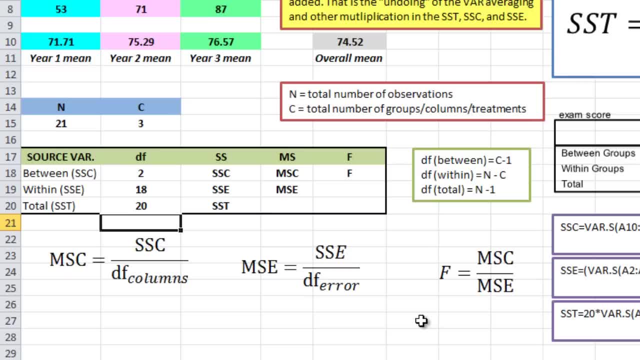 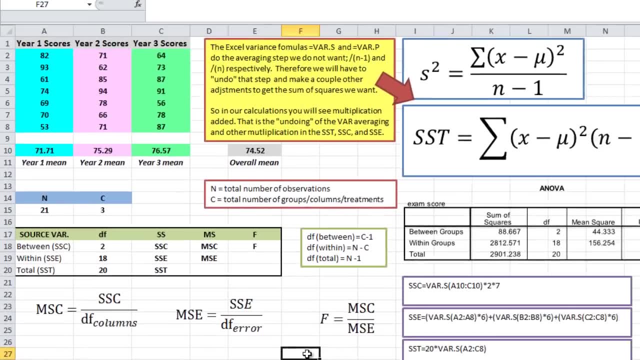 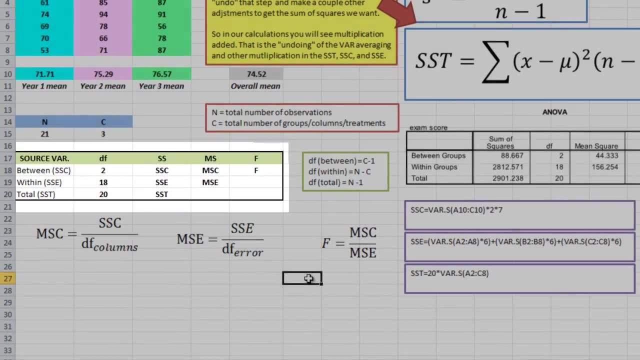 And that is 20.. So that's very, very easy. Now comes the hard part. Now we have to find the sum of squares. Now I went ahead and put placeholders in in our chart over on the left-hand side, so we know where everything goes. 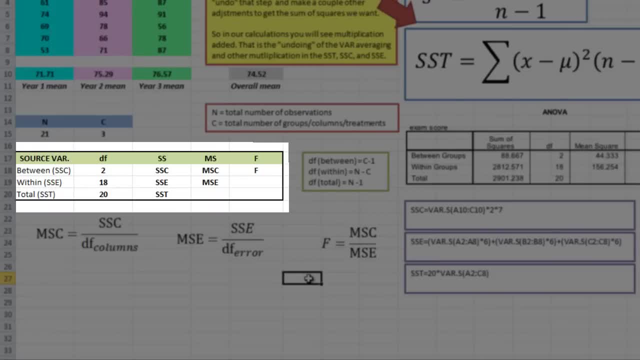 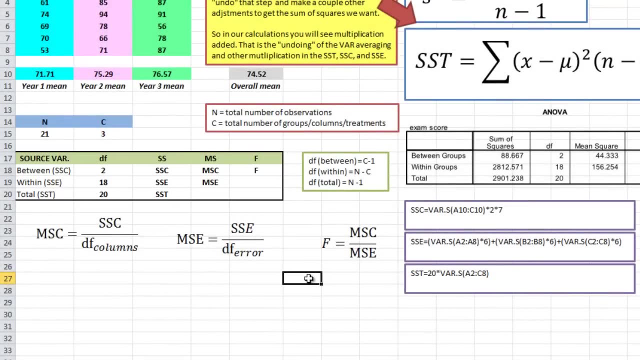 So if you look in the SS column we have SSC, SSE and SST Sum of squares column, sum of squares error and sum of squares total. Now on the lower right you will see boxes outlined in sort of a purple color. 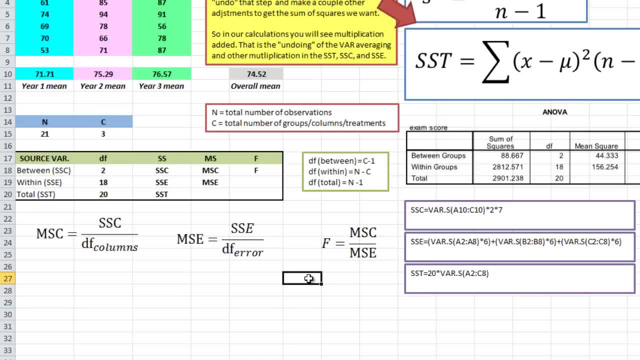 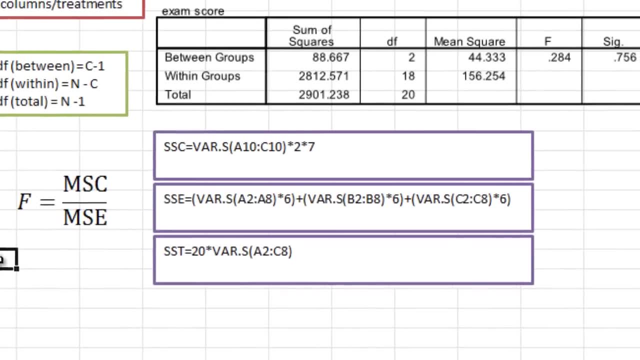 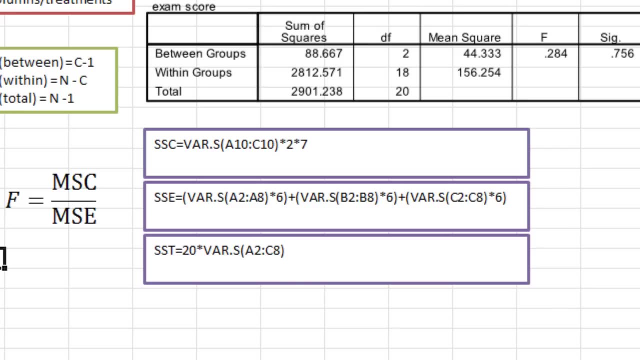 So those are the actual formulas we're going to put in each one of those cells. So let's take a look at each one very briefly Now. there might be some multiplication in here you don't fully understand, but you may not go over the actual formulas for SSC, SSE. 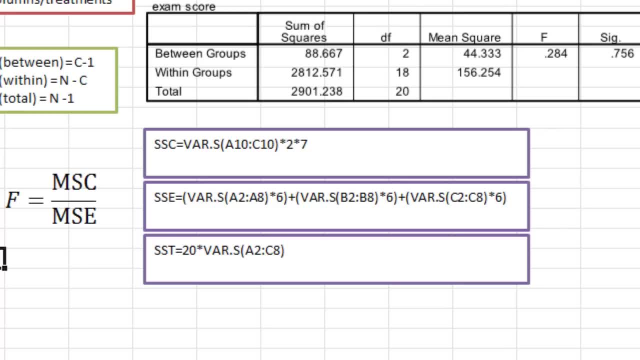 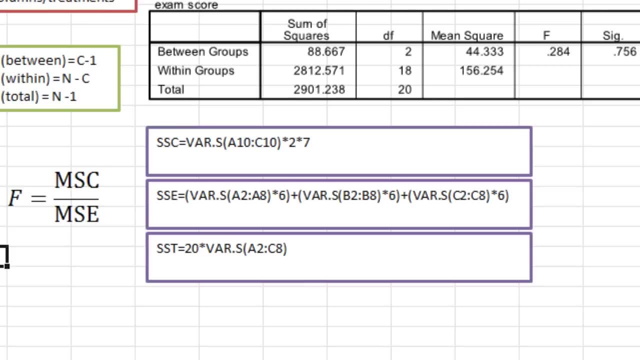 and SST because they are mind-numbing. You can find them in your book and the way we're doing it, you really don't have to worry about it. And that just sort of brings up my overall point: The chances of you having to do an. 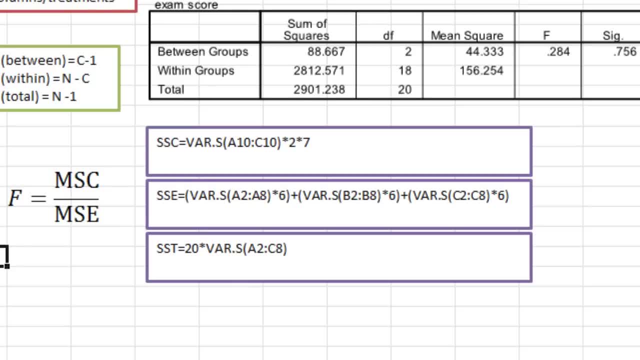 ANOVA by hand are basically zero. At least I hope not. You're going to be using Excel or SPSS or Minitab or whatever else it might be, So we're doing all this by hand, just so you can see how everything relates. 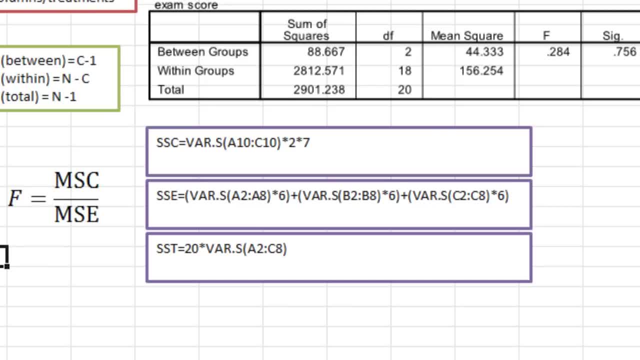 Because you'll have to do it that often, and hopefully never. So let's look at the top one first, And that is SSC. So in this one I'll go ahead and put my mouse in there. You can see that we have SSC equals. 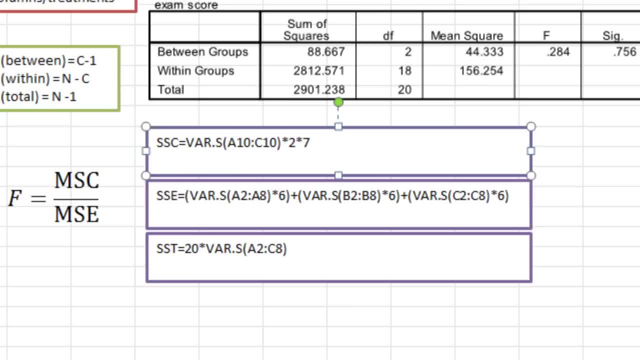 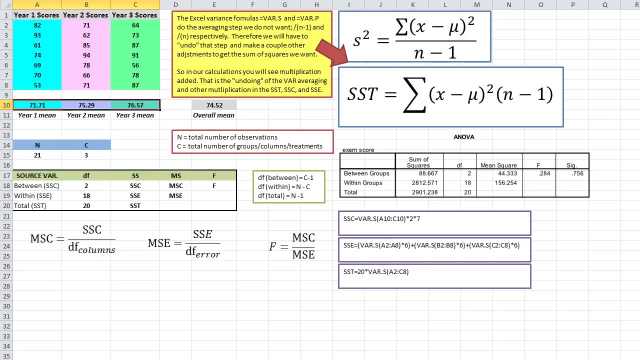 vars. that is the formula for sample variance And it's going to be cells A10 to C10.. Let's go up here: What is A10 and C10?? Well, that is the column means. So it's going to look at the variance. 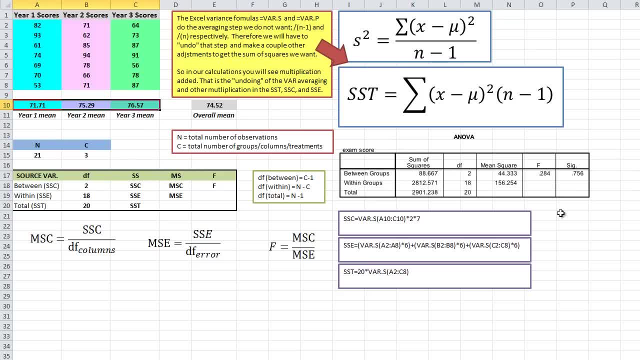 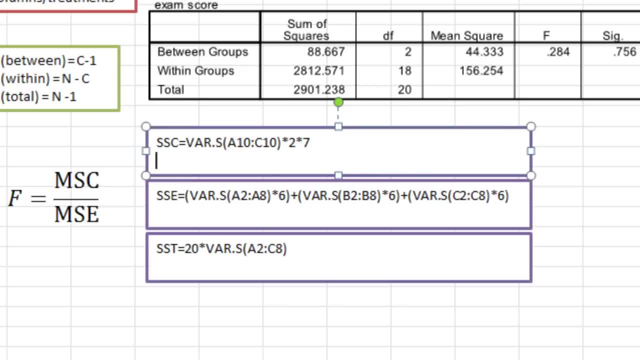 of those three column means, And then we multiply by 2.. Well, where does the 2 come from? In this case, the 2 comes from the number of columns we have minus 1.. So basically, that's the same way of saying its degrees of freedom. 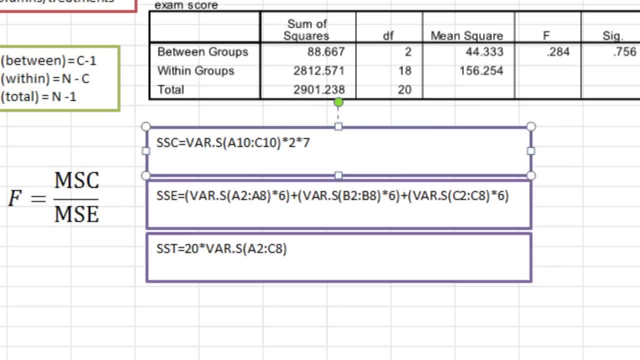 So that's where that 2 comes from. Where does the 7 come from? Well, that's how many observations we have in each column. So vars is the sample variance formula for those three column means Times 2, which is the number of columns minus 1. 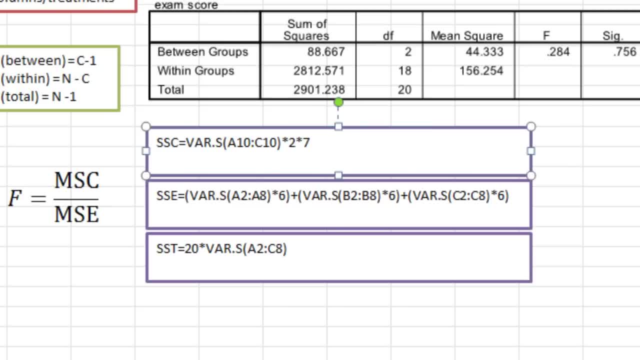 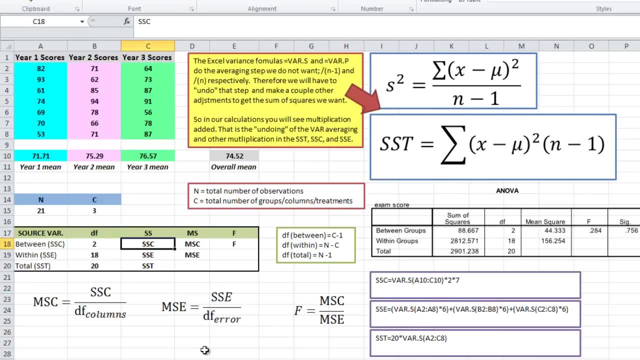 so that's 2.. Times 7, which is the number of observations in each column. So let's go ahead and go over here to our SSC box. I'm going to take out the text, Then I'm going to go over here and copy. 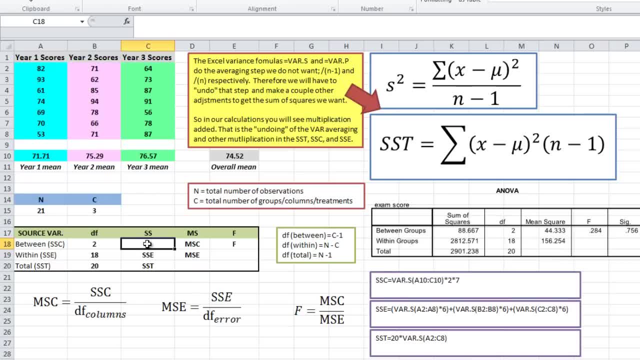 our text in our box. We'll go back over to the SSC cell. We'll paste it. Now I'm just going to take out the SSC part. So delete, delete, delete, Hit enter And there we go. So the sum of squares. 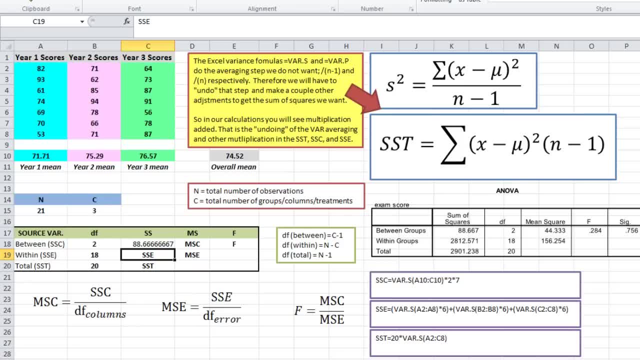 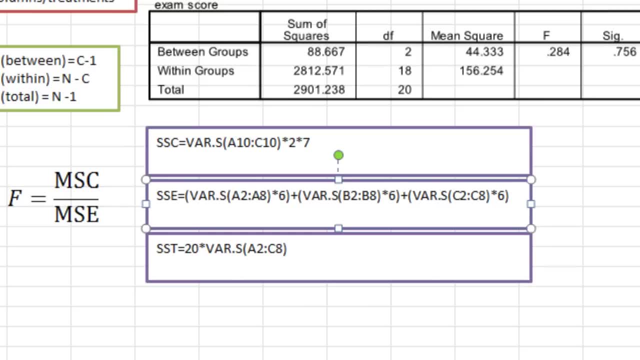 for the columns or the between sum of squares is 88.667 repeating. So now let's go ahead and look at the SSE formula, And it is admittedly much more involved, But if we take it apart, we can see where everything comes from. 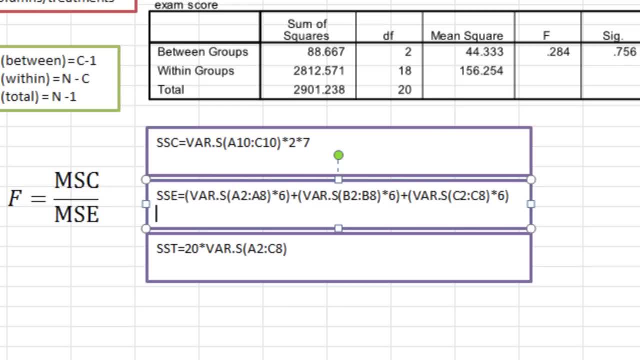 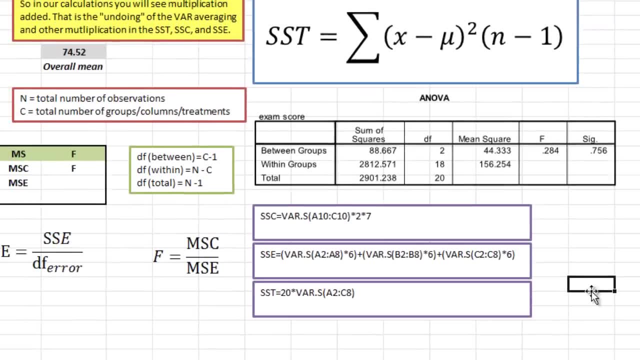 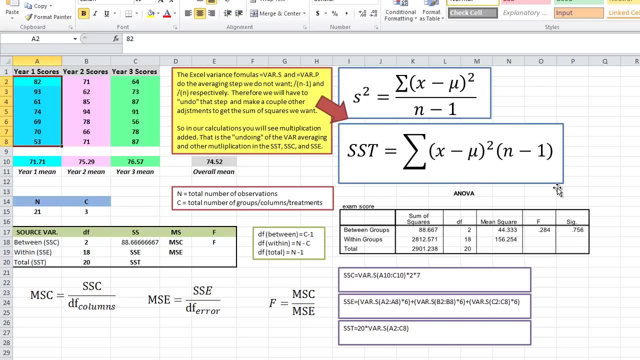 So we're using the vars formula again. So there's the sample variance. Now the first one asks for cells A2 through A8. Well, what are those? Well, A2 through A8 are the data points for column 1.. Or all the year 1 scores. 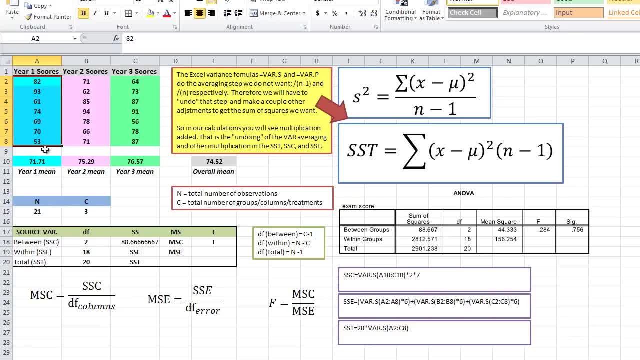 So we're asking for the sample variance of those 7 scores. Now we're going to multiply by 6.. Well, why are we multiplying by 6?? Well, that goes up to the formulas up here at the top. The sample variance is n-1. 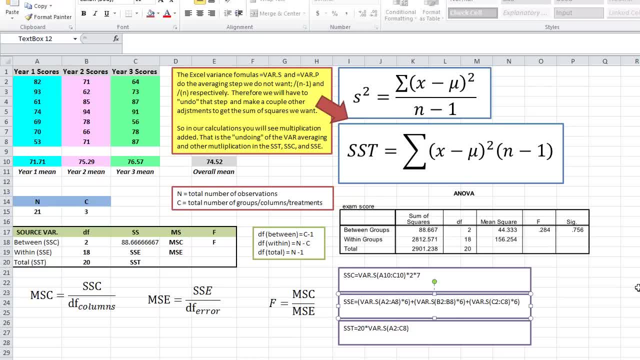 in the denominator. Well, we do not want that. We want to undo that. So that's why we're multiplying by 7-1, which of course is 6.. Then we're going to add to that the variance of the next column. 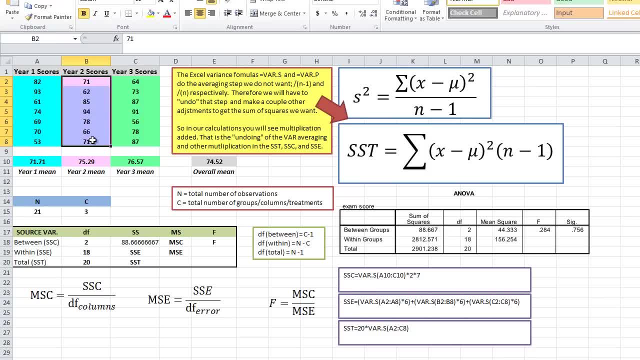 So B2 through B8, same thing times 6.. And then we're going to add that to the variance for 3.. So C2 through C8.. So that is all that is. It's just the variance of each column added together. 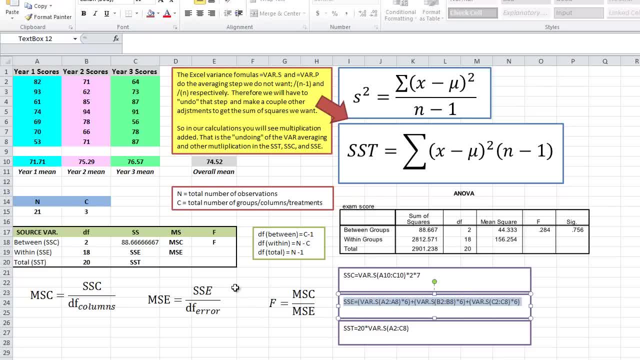 So we'll go ahead and copy all that, But first we'll go over to SSE and delete it. Make room. Now we'll go over, copy all that, Control C on my PC, Control V to paste it. Now I'm going to go up and modify it by taking out the 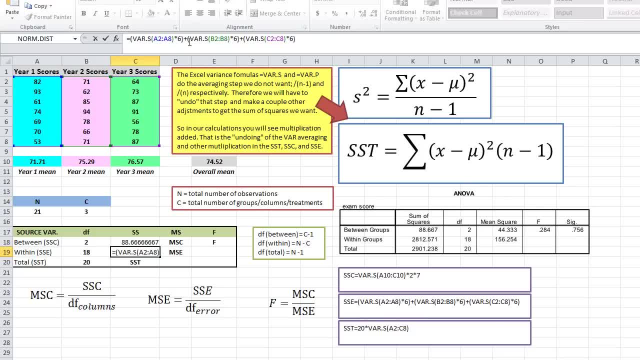 SSE at the beginning: Delete. Then we'll hit enter And there we have a sum of squares within, or an SSE of 2812.57. So that is our sum of squares of the within, And again that's within the columns. We just add them all together. 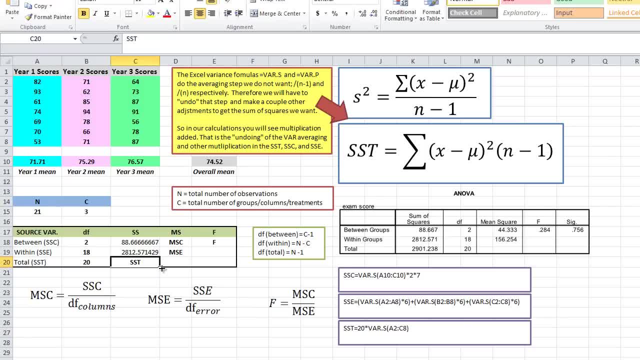 Now we'll go to SST- sum of squares, total. So we'll delete that. If we look down here in our formula we have: SST equals 20 times var s of A2 through C8.. Well, what is A2 through C8? That's. 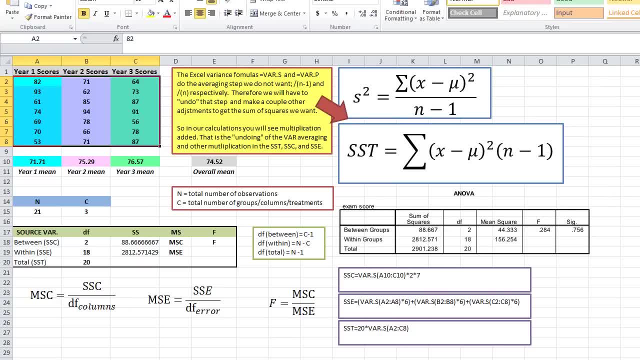 everything. So A2 through C8 is our entire data set. Now we take the variance of that and we multiply it by 20.. Why? Well, remember, our variance is N minus 1.. So we have 21 scores minus 1.. We're going to need to undo. 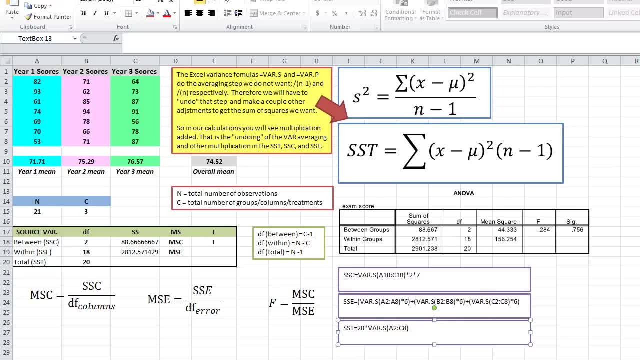 that put it in the top. So that's what we multiply by 20.. So we'll go ahead and select all that Control C to copy. We'll go over to our SS column here the SST Control V to paste. 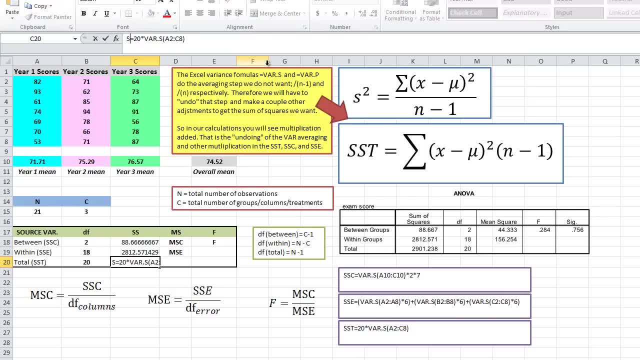 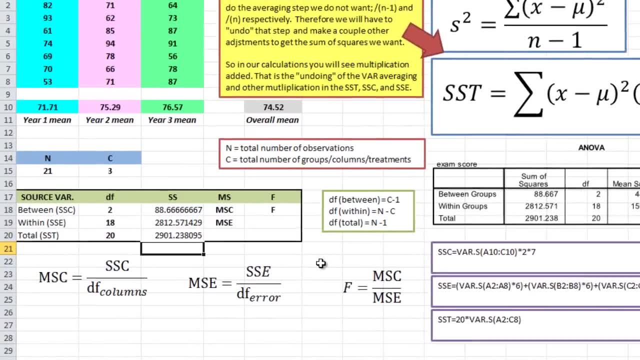 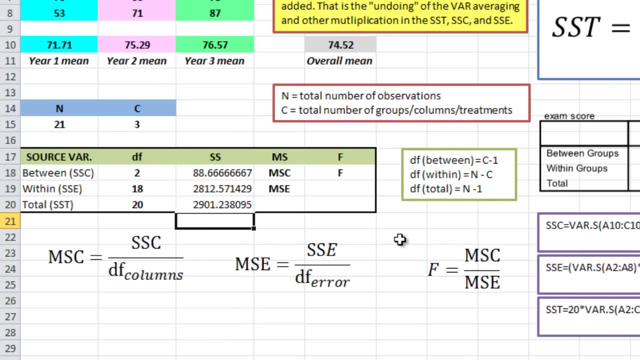 We'll take out the SST at the beginning. Hit enter and there we go. Now, if you look close enough, you will see that the SST is the sum of the SSE and the SSC, So 88.6667 plus 2812.57. 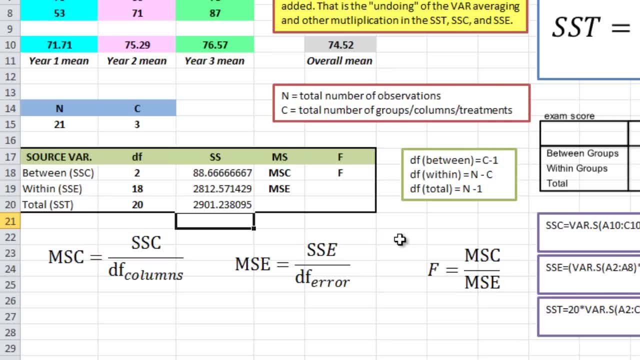 ish. When you add those together you will get 2901.23.. So that goes back to the idea of partitioning the total variance. So our total variance of SST is made up of two components: the SSE and the SSC. 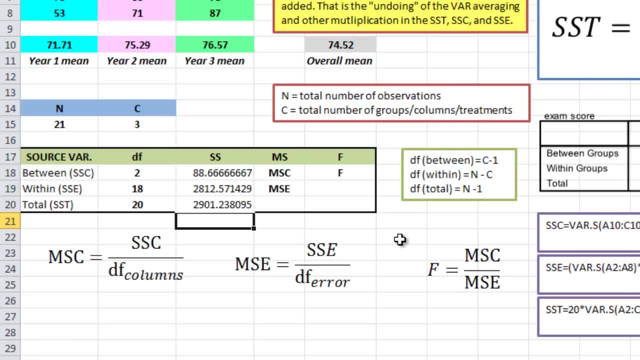 When you add those together, you get the SST in return. Okay, so a few more things to do. Now we need to find the MSC, So that's up here under the MS column. Now, if you look down here, I have a little formula for. 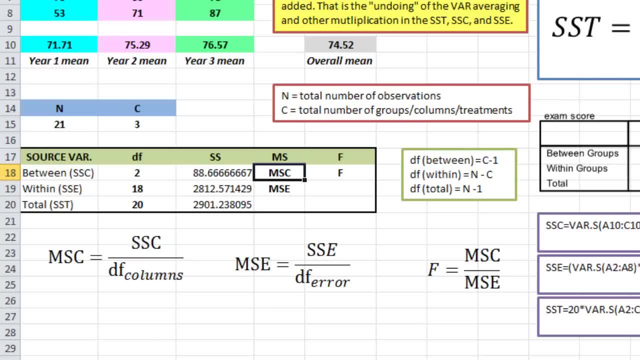 the MSC, or the mean square of the columns. So we're going to delete the text And this is just the SSC divided by the degrees of freedom for columns, And we have both of those. So this is equal, the SSC which we just found, which is over here. 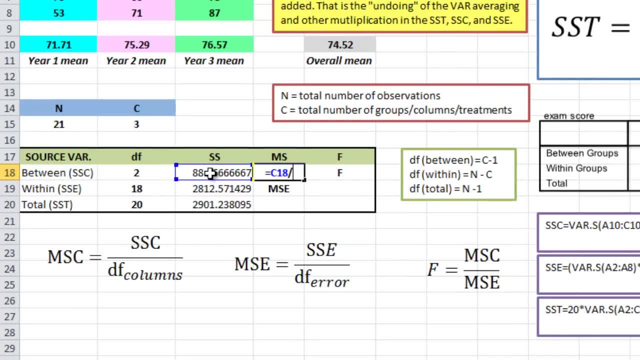 divided by the degrees of freedom for the SSC, which is to the left of that. So we go ahead and click that cell and hit enter. Now we have a mean square for the columns of 44.3333, repeating. Now let's go ahead and do the MSE. 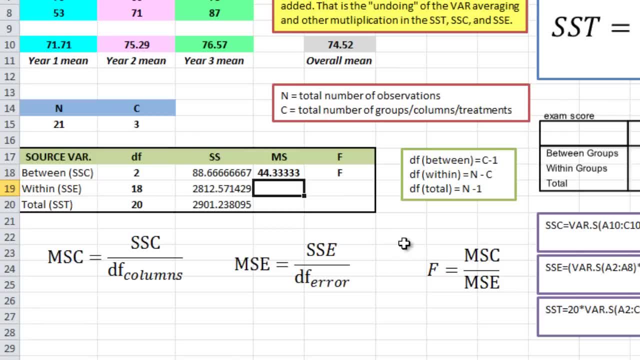 So we'll delete the text. and that's the SSC. So this is the SSE divided by its degrees of freedom. So we'll go to that cell we already have selected. This is equal, the SSE, the 2812.57 or whatever it was. 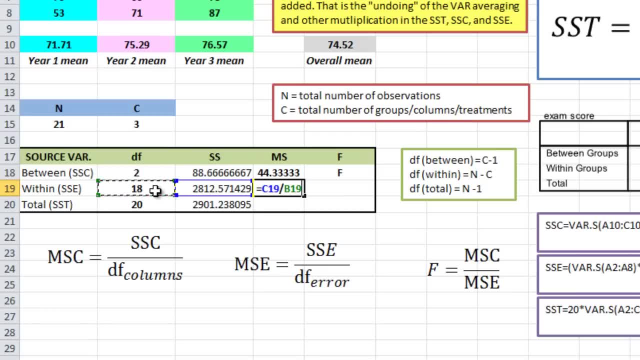 divided by its degrees of freedom, which is to the left of it, That's 18.. And we'll go ahead and hit enter, And that is 156.257.. So now we have our MSC and our MSE. Now what is F? 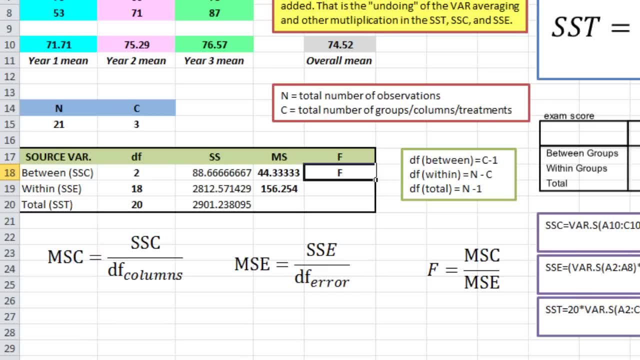 Well, F is merely division, The MSC divided by the MSC. Of course we have both of those, we just did them. So the F here equals the MSC which is there to the left, divided by the MSE we found Which is there. 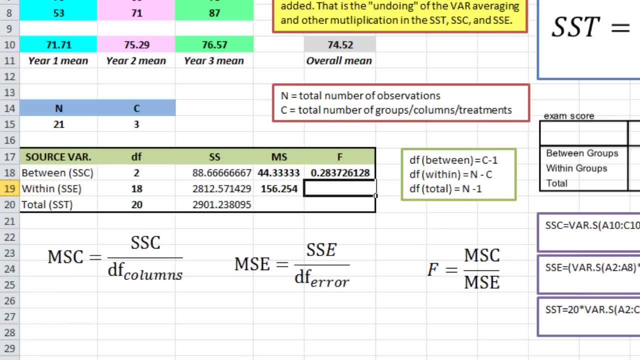 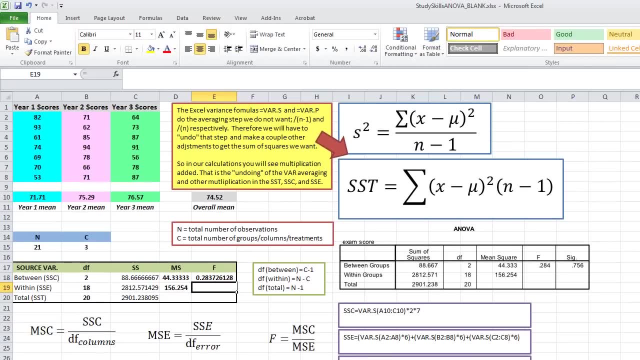 Hit enter And you'll notice we have .283726, etc. What was it? SPS output. Look over here on the right: Our F is .284.. Same thing. So look at the SPSS output over here on the right and our chart we just did over here. 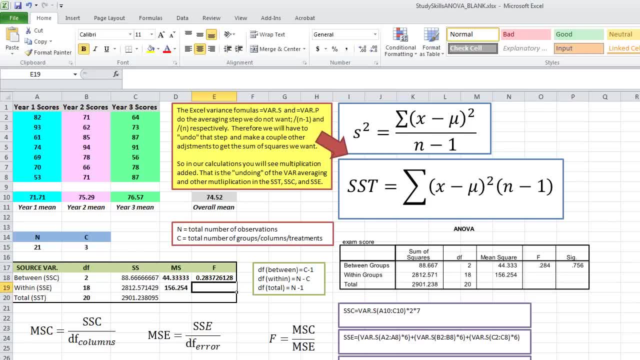 on the left. What do you notice? Degrees of freedom for the between groups is 2.. Degrees of freedom for the within is 18.. Degrees of freedom total is 20.. The sum of squares for the between is 88.667.. It's in both. 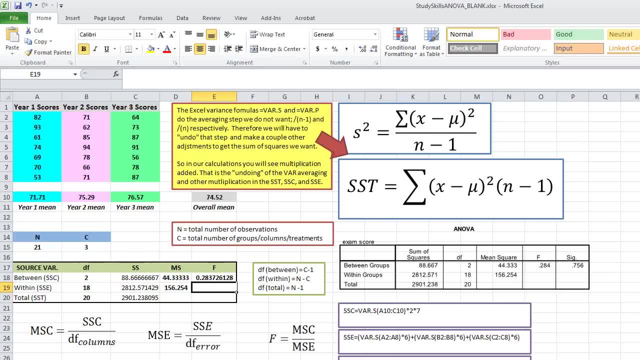 The within sum of squares was 2812.57, Same in both. Sum of squares total 2901.238, Same in both. So in Excel, by hand, we just replicated the output SPSS gave us. So now you can see how everything works together. 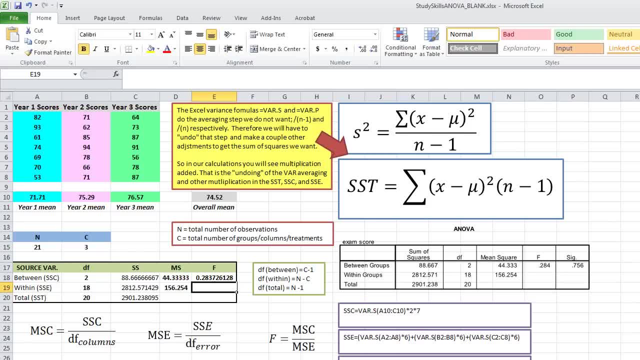 Now, of course, I do admit, the only odd part of this are these formulas down here, And again you're just going to have to look at them and figure out where everything is being pulled from. But you're very smart and I know you can do that. 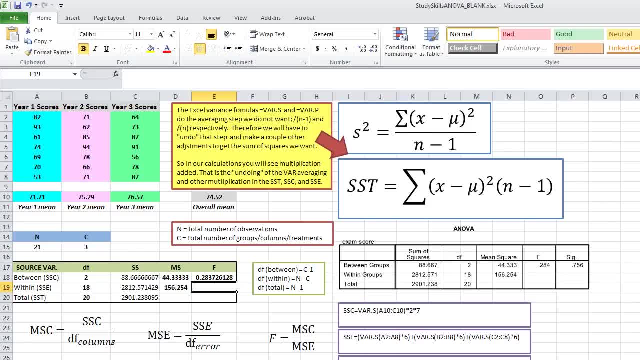 So let's do one more thing and let's actually use Excel's built in ANOVA to see if we get the same thing. So we're going to go ahead and go up to data here at the top of the ribbon, Go all the way over to 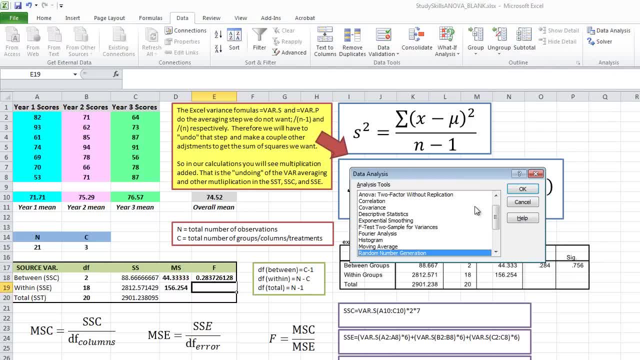 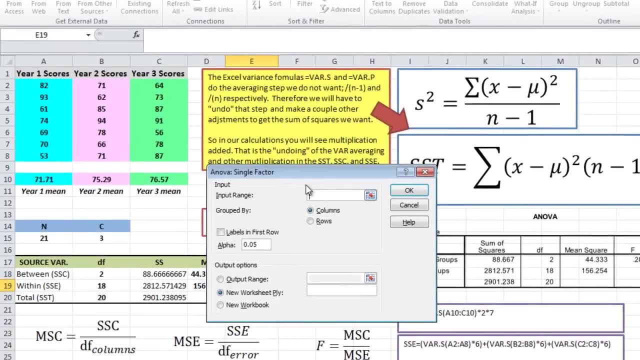 the right and you'll see data analysis. So we'll click on that Now. remember we are doing the ANOVA single factor, So go ahead and click on OK. Now this wants the input range, So we'll select the little icon on the right. 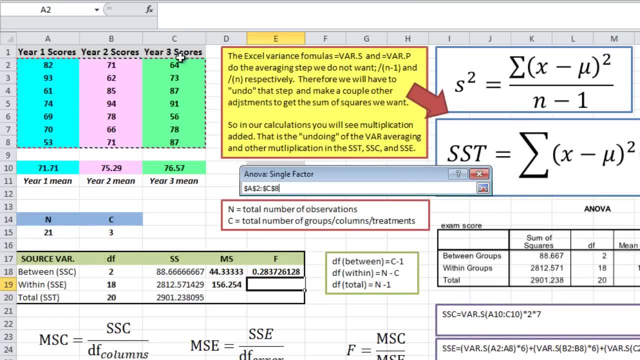 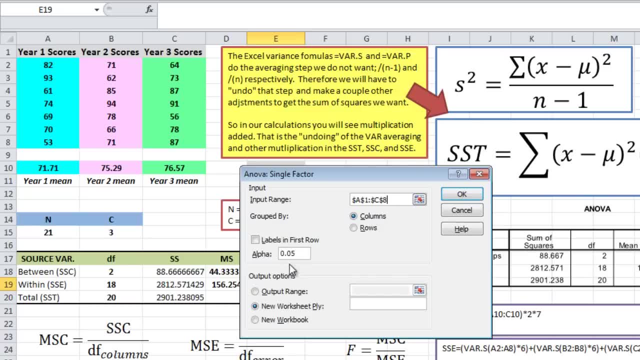 and then we'll select all of our data, And actually I'm going to select the column headings too. We'll go back. It's grouped by columns. We have labels in the first row. Our alpha is .05.. We're going to stick with that. 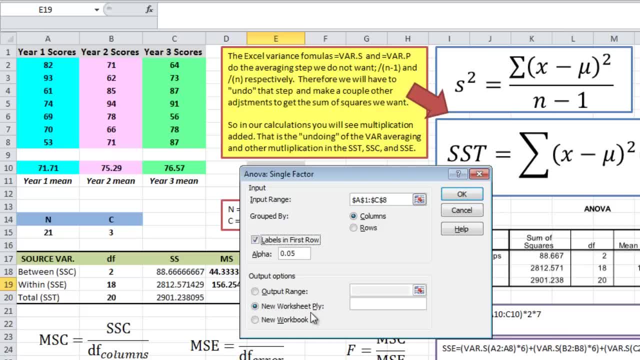 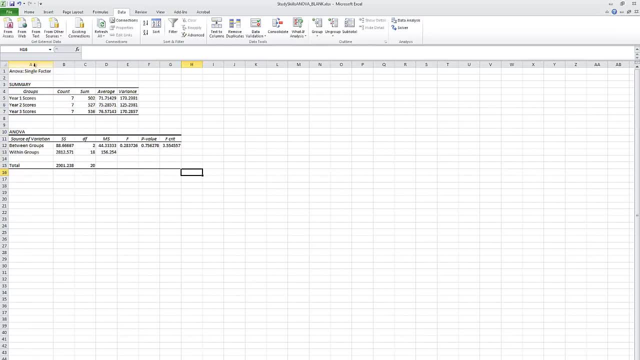 And we'll leave it to new worksheet ply. Those will give us all of our results on a new worksheet. We'll go ahead and click OK, And here we go. So I'm going to go ahead and spread some of these columns out. 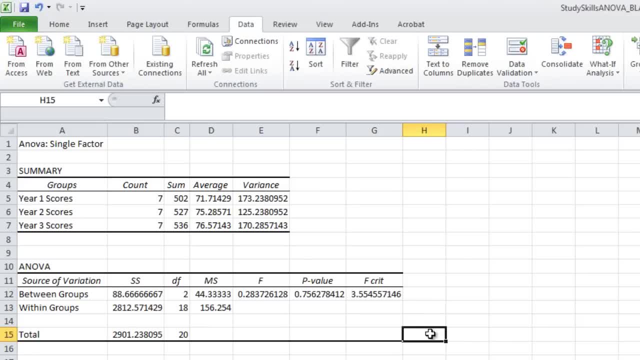 OK, Now a few things to look at- Actually a lot to look at. So you can see that we have a summary of each score group. So year one students, year two students and year three students. So it gives us our count. 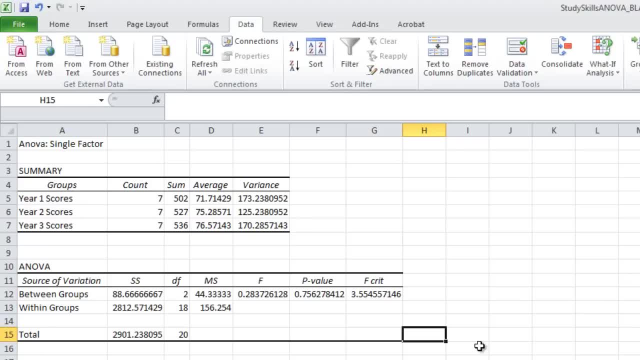 the sum of all those, the average and the variance in each column. So we'll go down to the bottom. That's our actual ANOVA table. So you can see our between group sum of squares: 88.6667.. 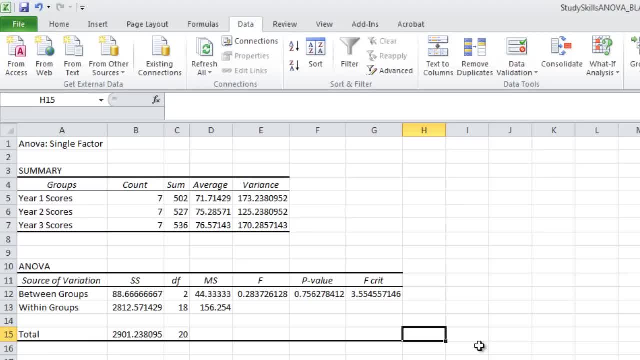 Same thing Within groups: sum of squares 2812.57.. Same thing: Total sum of squares: 29.24.. Same thing, Degrees of freedom: 218 and 20.. Good, Our mean squares for the between or the columns, 44.33.. 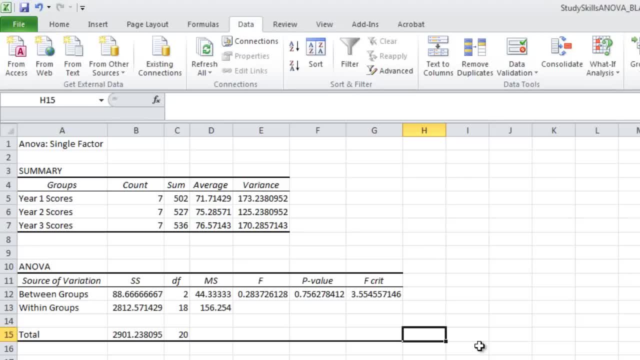 Good, Our within mean square 156.25.. Very good, Divide those. We have an F of .2837, etc. Same thing we had before. Now this gives us a few more bits of information which are helpful. Now remember that when we're doing. 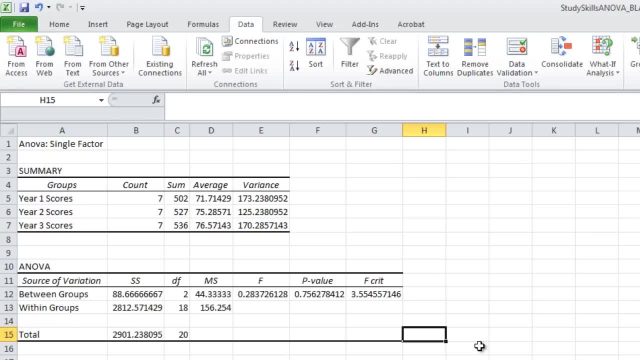 this sort of problem. we're going to test our F value of .2837 against an F critical value in the F distribution, based on our degrees of freedom in the numerator of 2 and degrees of freedom of 18 in the denominator with an alpha of. 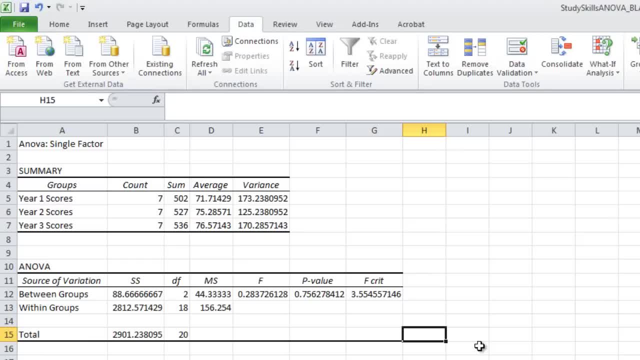 .05.. We learned how to do that a long time ago, So our F critical is 3.5545.. So is our F statistic of .2837 larger or beyond 3.554?? Well, no, So we would fail to reject. 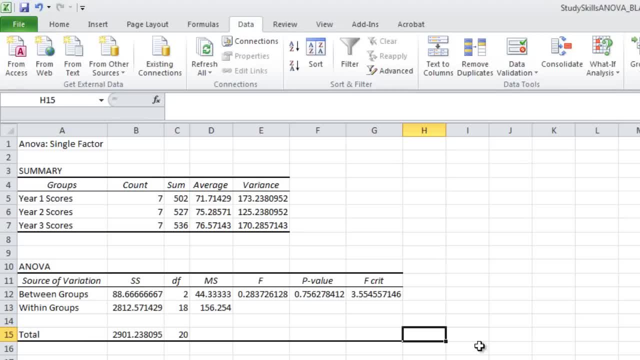 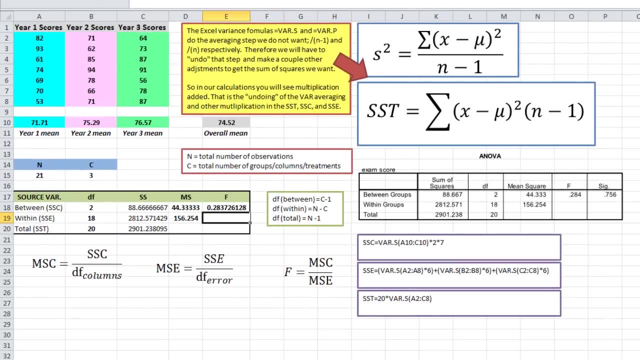 our null hypothesis that these three means are different. So let's go back to our original And you can see that all this is the same now. So our SPSS output we set out to replicate. we did by hand over here on the left And we did it. 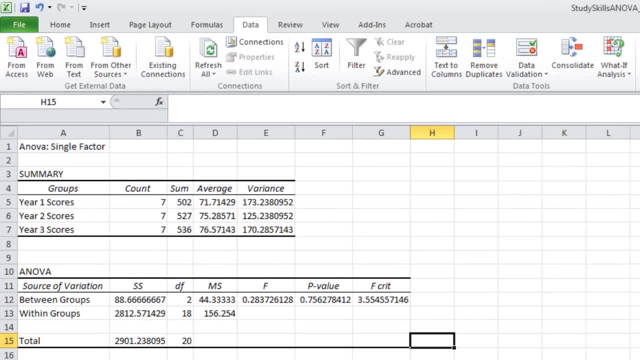 in Excel, using its built-in formula. Now, of course, that's the whole point. We will not do this by hand. We will either use Excel or we'll use some other statistical package, But I wanted to show you where all this information. 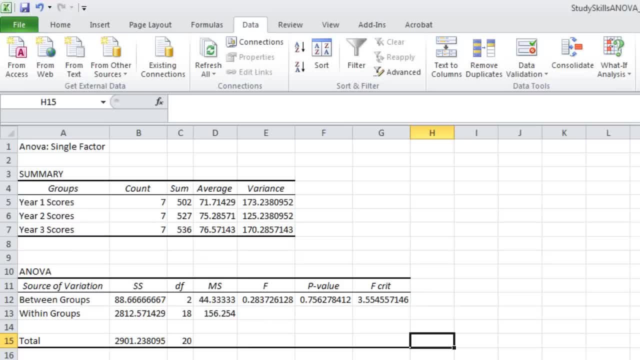 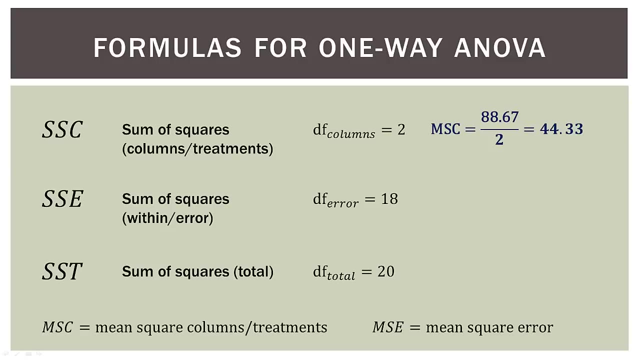 comes from, so you can understand the foundation sort of the guts, the workings, the gears of the ANOVA process. So let's go ahead and go back into PowerPoint and finish everything up. Let's go ahead and put in our numbers from Excel. 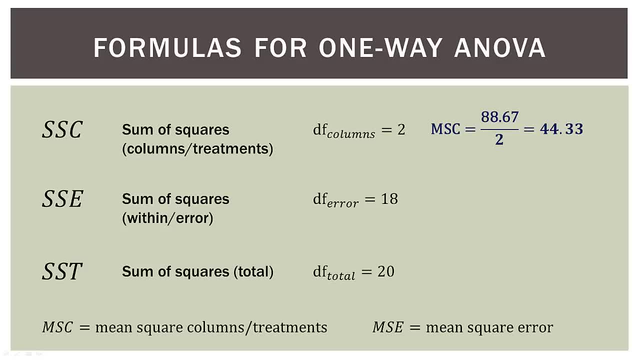 So remember, in Excel we found that the SSC, or the sum of squares in the columns, was 88.67.. Then we divide that by our degrees of freedom, which is 2, and we end up with an MSC of 44.33.. Now 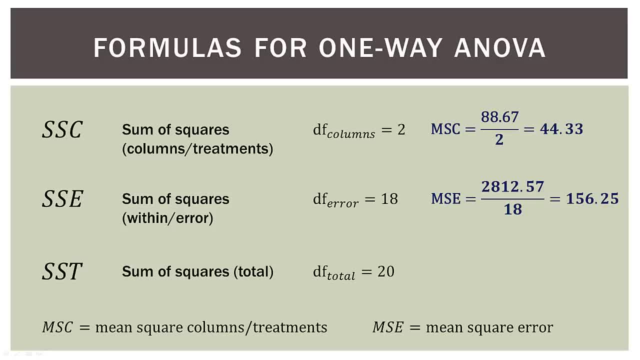 the MSE is the SSE divided by 18.. So that was 2812.57 divided by 18.. And that comes out to an MSE of 156.25.. So remember our F ratio. here is the MSC divided by the MSE. 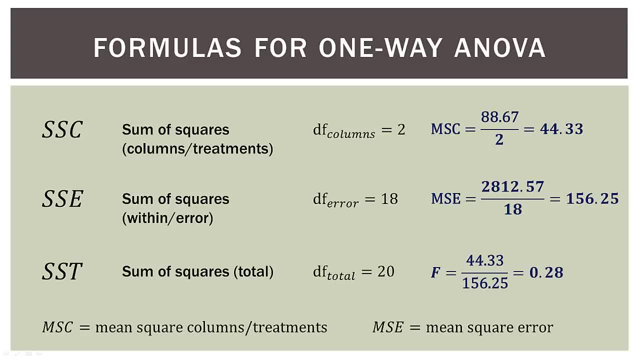 So the mean squared of the columns divided by the mean squared of the error, Or you can think of it as the mean squared between divided by the mean squared within. So that is 44.33 divided by 156.25.. And we end up with an F statistic. 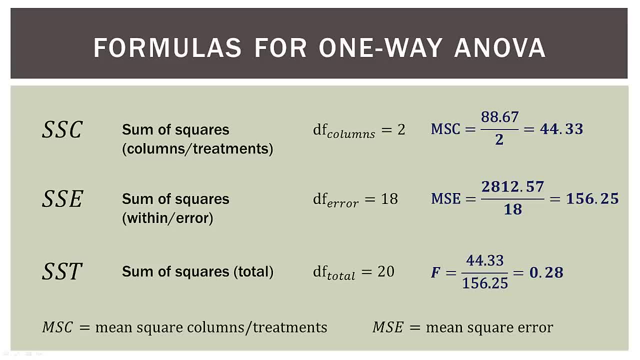 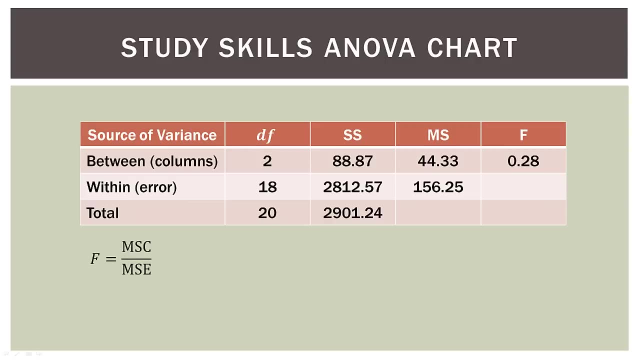 of 0.28.. And that is exactly what SPSS gave us and what Excel's own built-in ANOVA calculator gave us as well. So we know we did it correctly Now, how do we ultimately interpret this? So our 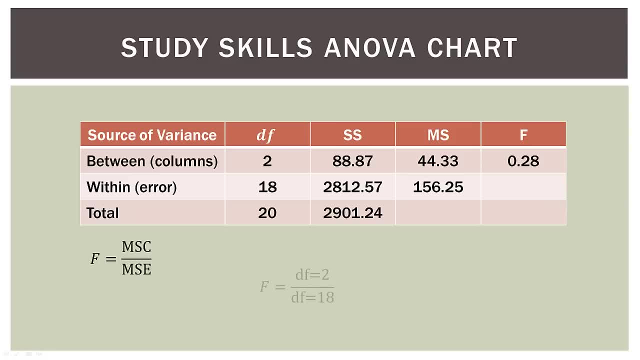 F ratio is the MSC divided by the MSE. That's what we just did. Now, in the numerator we have a degrees of freedom of 2 and in the denominator we have a degrees of freedom of 18.. So remember, when we look up a critical. 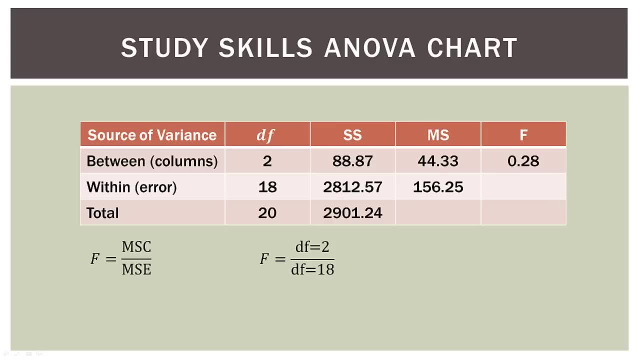 value. in the F distribution we have a numerator- degrees of freedom- and a denominator- degrees of freedom- And in this case those two degrees of freedoms come from our formulas for the MSC and the MSE. So we can write this F statistic we gotta find. 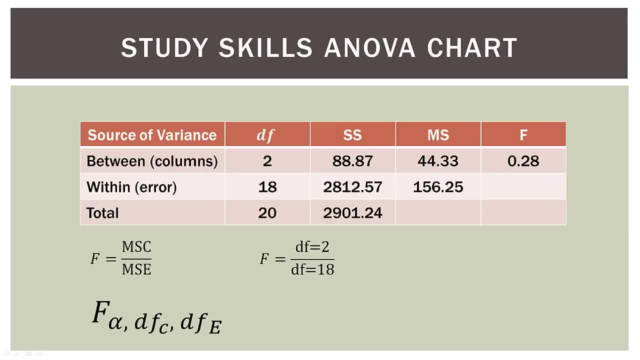 like this. So we have an alpha level, say 0.05, then we have degrees of freedom of C, the columns, and degrees of freedom for the error E. So that is, degrees of freedom in the numerator and the degrees of freedom in the denominator. 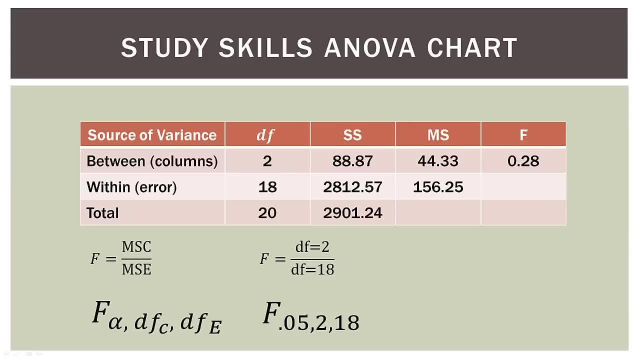 So we can write it like this: So we need to find the critical value of F with an alpha of 0.05, a numerator degrees of freedom of 2 and a denominator degrees of freedom of 18.. And we already learned how to do that in a previous. 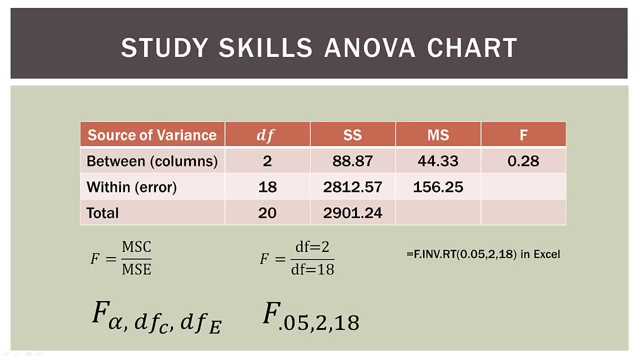 video. Now, the easiest way is to go into Excel and use the F, dot, INV, dot, RT function. that's the F distribution, the inverse right tailed. that's what all that stands for and we put in those three parameters. So an alpha of. 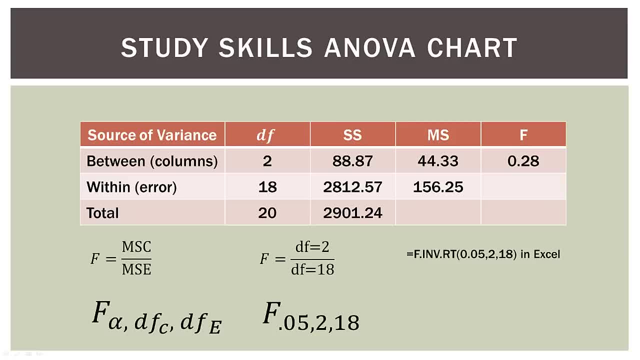 0.05, a numerator degrees of freedom of 2 and a denominator degrees of freedom of 18.. So when we put that into an Excel cell we will get an F critical value of 3.55.. So we have to ask. 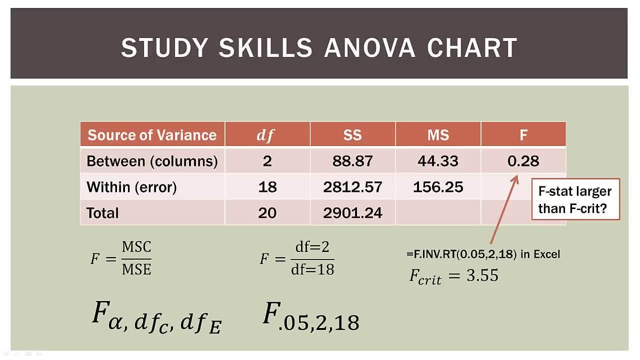 ourselves. is the F statistic in our ANOVA table larger than our F critical value? Well, no. So remember what our null hypothesis said. We talked about this in the first ANOVA video And these type of problems, our null hypothesis. 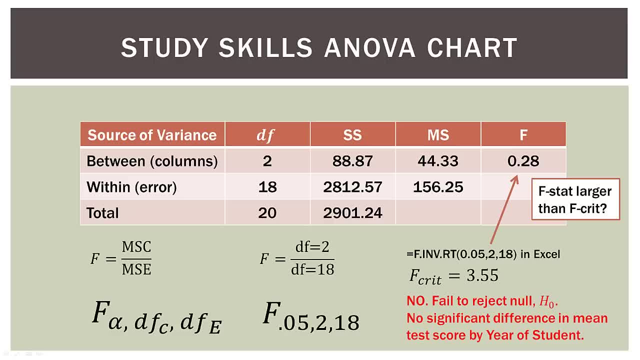 is that the means are equal to each other. That's another way of saying that the means, the three means, come from a common population. So since our F statistic is so low and does not exceed the F critical value, we fail to reject our null. 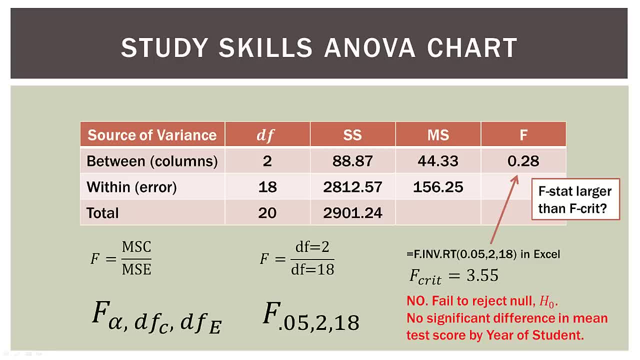 hypothesis. So we found no significant difference in mean test score by year of student. So the means of the first year students, the second year students and the third year students on their study skills exam did not differ significantly, And that's it. 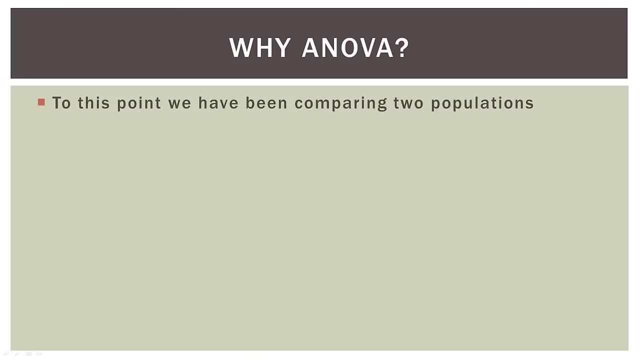 So remember, up to this point, we could only do comparisons involving two populations: Independent sample t-test and match sample t-test. Limiting ourselves to those two comparisons is, of course, limiting. What if we wanted to compare the means of more than two populations? 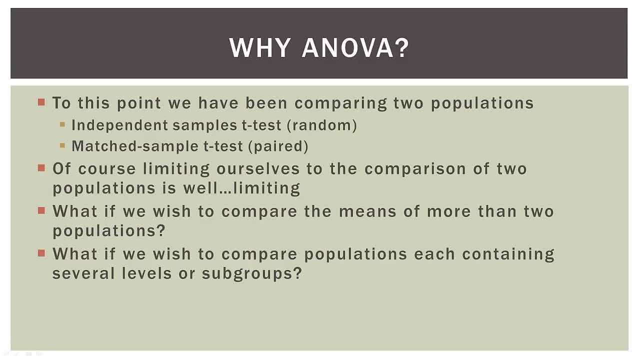 like we did in this problem. What if we wanted to compare the populations, each containing several levels or subgroups? So this hints at the two-way ANOVA. So imagine a scenario where we have your one students, your two students. 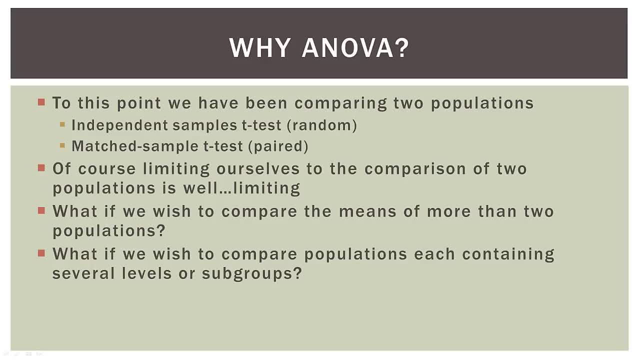 and your three students, But on the other axis we divide them into male and female. Now we have two factors, So our first factor is the year of the student And our second factor is their biological sex. That would be a two-way ANOVA. 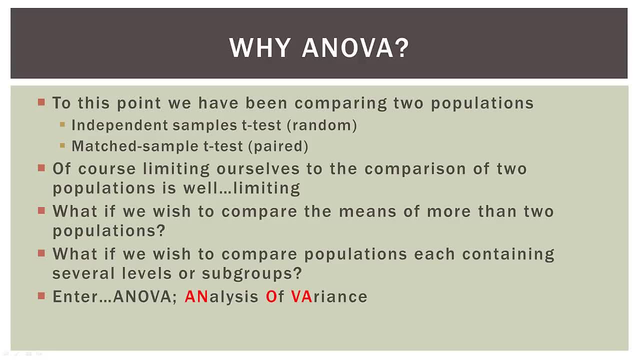 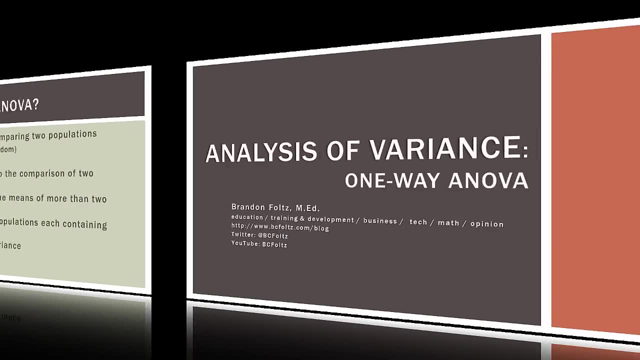 And we can do that, of course, using this technique. So the analysis of variance is the tool we use to do those more complex analyses. Okay, so that wraps up part two of our video on the one-way ANOVA, or the 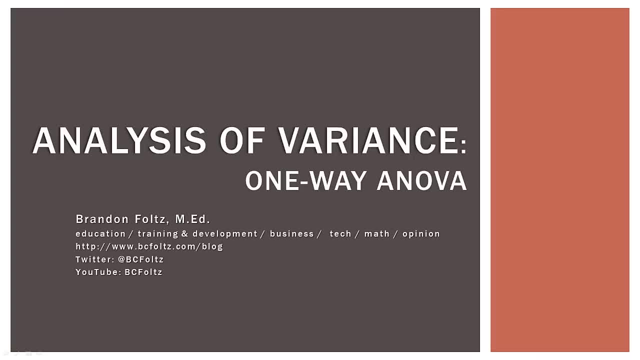 one-way analysis of variance. Now, I know it was a lot to digest, But I really wanted to take you from the very basic conceptual foundations up through an example problem so you can see how all the data is related to each other. learn how to do the sum of squares. 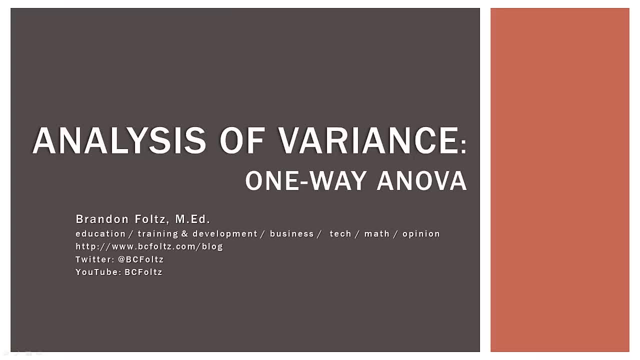 and then eventually find the relationship between those sum of squares, because that is the foundation of how we conduct the ANOVA. So I have no doubt that you may need to go back and watch parts of the video to really grasp it, But hopefully after watching. 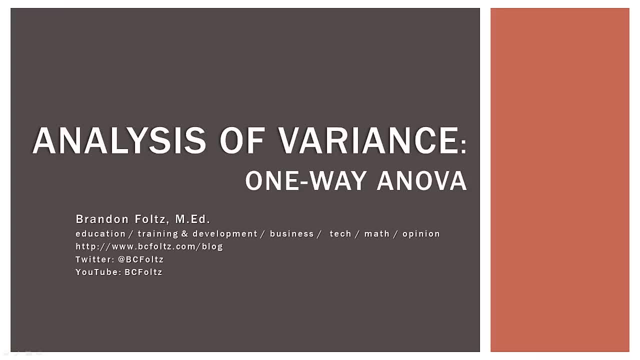 it, you have a really good, solid understanding of what ANOVA is. So a few reminders and then we're done. If you're watching the video because you're struggling in a class, stay positive and keep your head up. You're an amazing, smart, talented. 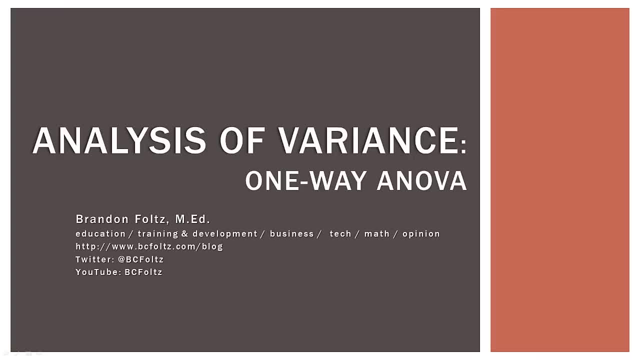 person. Never let anyone tell you any differently, including yourself. If you liked the video, please give it a thumbs up, share it with classmates or colleagues or put it on a playlist. Feel free to follow me here on YouTube, on Twitter.